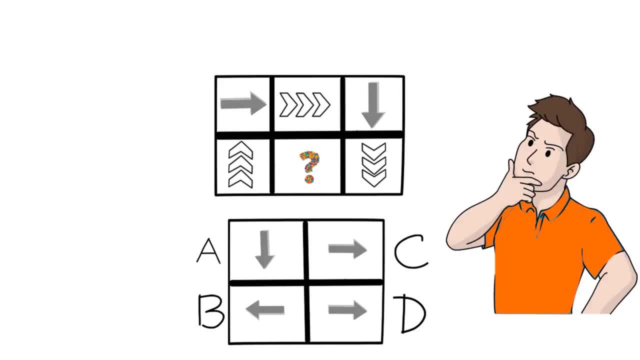 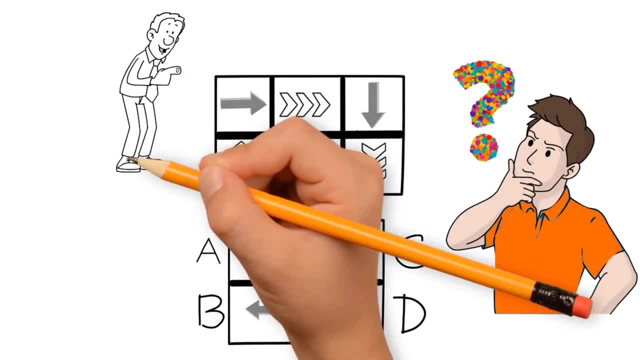 15 seconds to see if you can identify the right answer. Did you figure out the correct answer? Let's continue to see if we can get to the correct solution together. To solve these types of challenges, you always need to look for patterns, And there are three different. 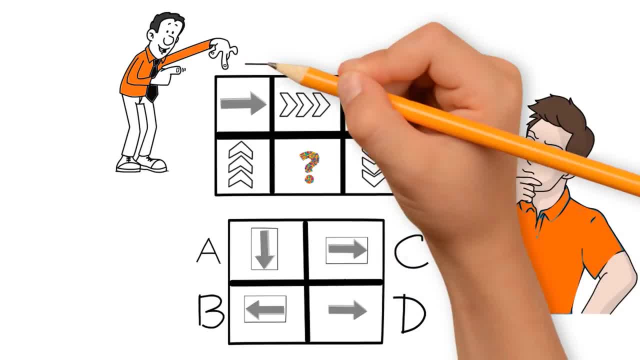 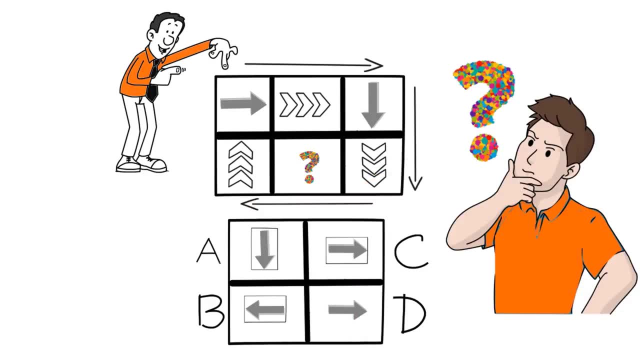 choices. One is missing, The other is missing, The third is missing, The fourth is missing. Patterns present in this sequence. Let's look at the pattern one. If we start from the upper left corner and go clockwise, you see that the arrows change alternatively in each subsequent box. 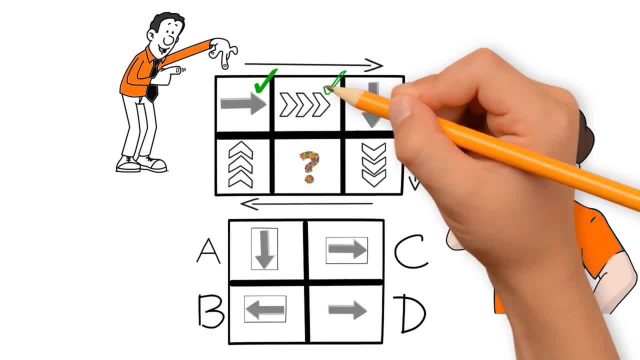 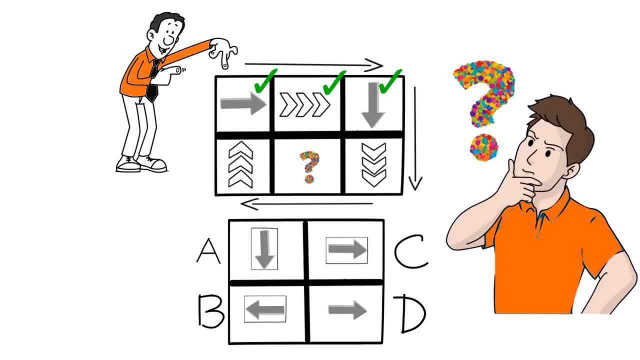 Second pattern is that inside the box, solid arrows rotate clockwise. And then the third pattern, which is a little harder to identify, is that the previous arrow points to the next arrow start. This is why the missing part, the part that you would need to identify. 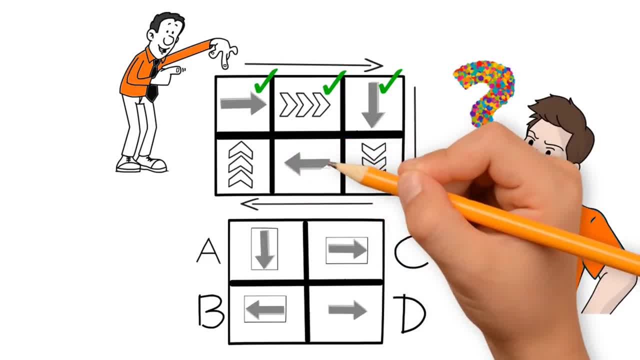 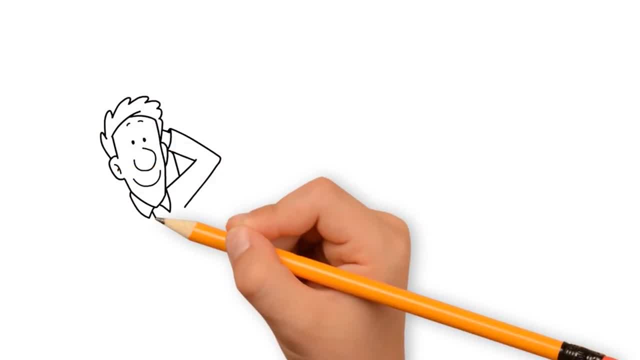 contains an arrow placed in the right corner pointing to the left, So the correct answer here is choice B. Hopefully you've nailed this question and now know how to answer similar problems in the test, But in case you need more problems and solutions, please make sure to check. 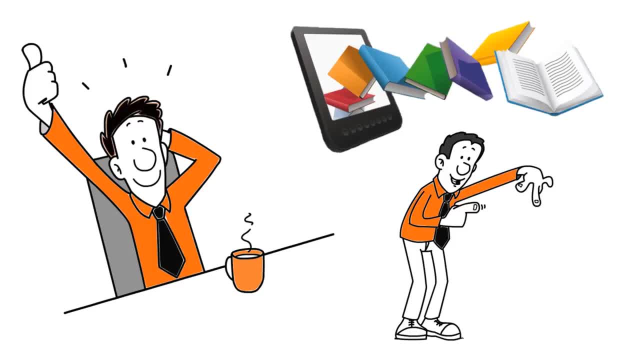 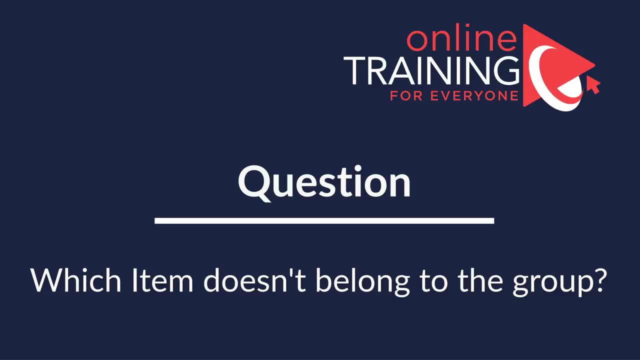 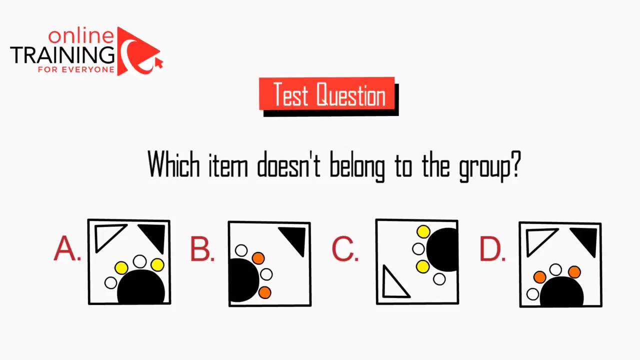 out my ebook. in the description section of this video, The types of questions you're looking at is very frequently used in the test. Typically, you're being asked to determine the answer to the question. You need to determine the item which does not belong to the group And you're presented. 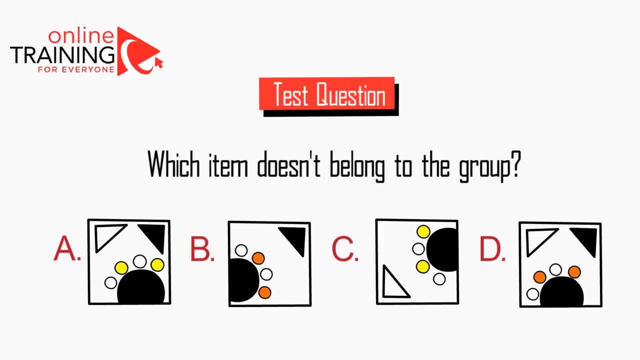 with multiple items. In our choice, we have choices A, B, C and D. Each item is represented as a square which contains multiple different items inside, And you need to determine the item which does not belong to this particular pattern or sequence. Do you see the answer? Please take a. 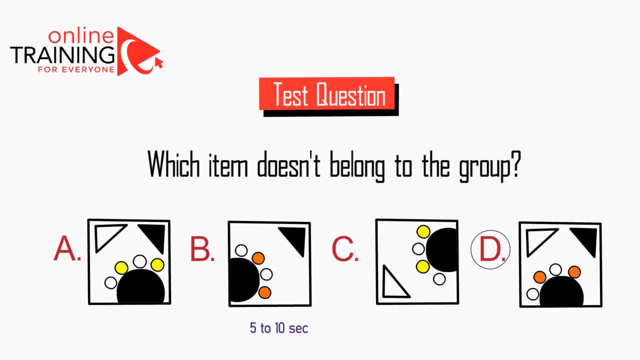 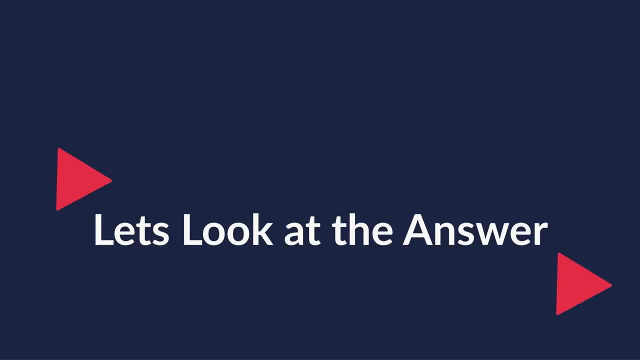 look to see if you can come up with the solution. 5 to 10 seconds, Maybe 10 to 20 seconds to see if you can come up with the answer. Did you figure it out? Let's continue to see how we can go and get to the correct solution together, As you might. 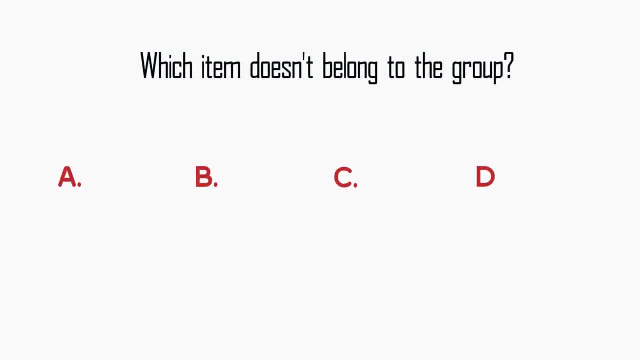 have figured out by now. there is always a pattern that you need to detect to answer these types of questions correctly, And a lot of times there are items that are designed to confuse you. So let me first walk you through the items that are designed to confuse you. You have small circles. 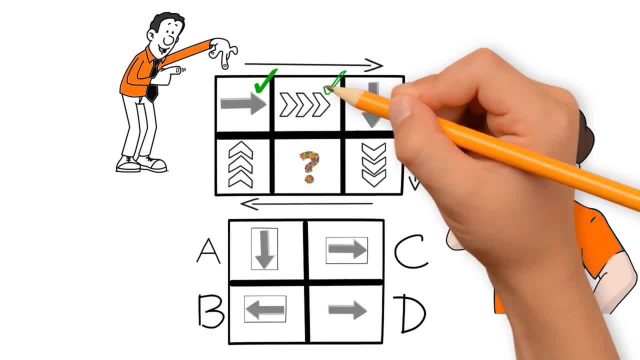 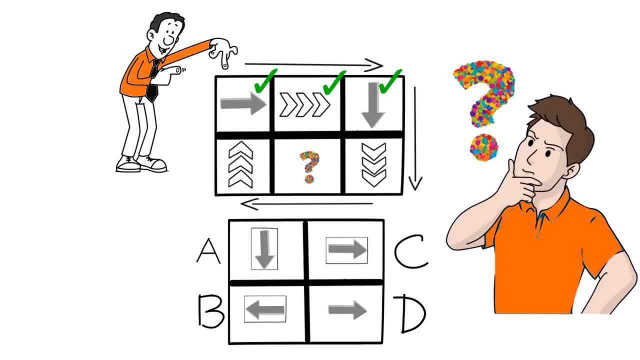 Second pattern is that inside the box, solid arrows rotate clockwise. And then the third pattern, which is a little harder to identify, is that the previous arrow points to the next arrow start. This is why the missing part, the part that you would need to identify. 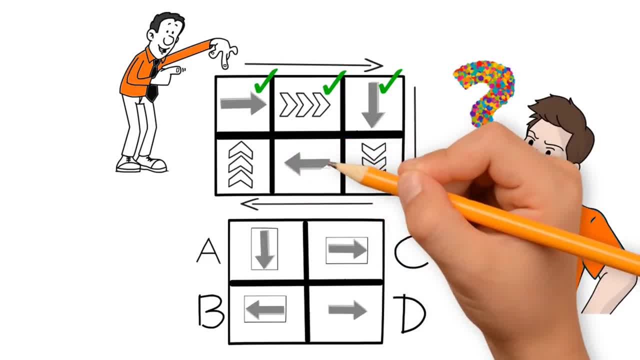 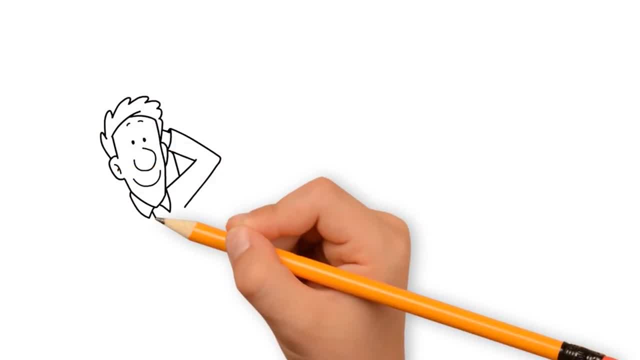 contains an arrow placed in the right corner pointing to the left, So the correct answer here is choice B. Hopefully you've nailed this question and now know how to answer similar problems in the test, But in case you need more problems and solutions, please make sure to check. 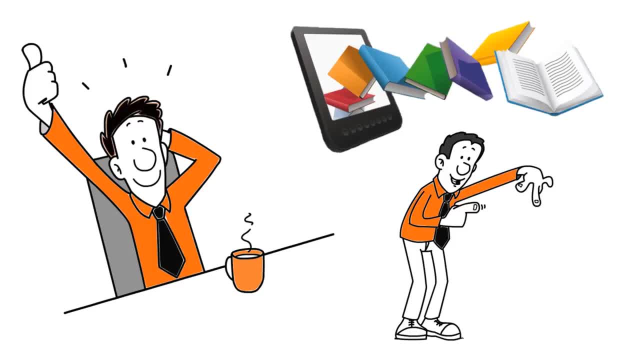 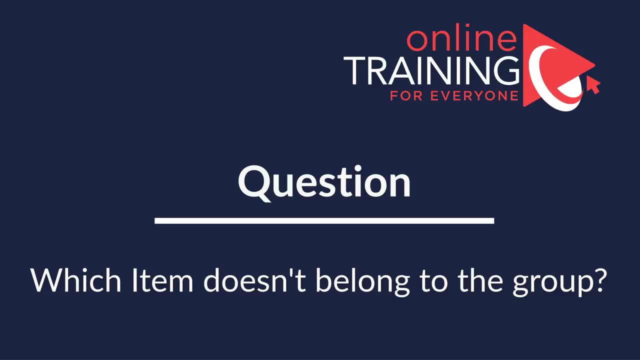 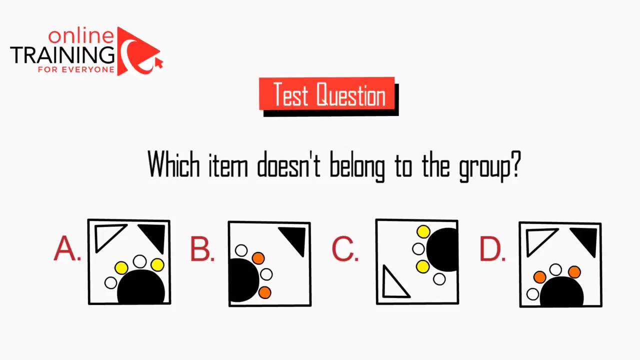 out my ebook. in the description section of this video, The types of questions you're looking at is very frequently used in the test. Typically, you're being asked to determine the answer to the question. You need to determine the item which does not belong to the group And you're presented. 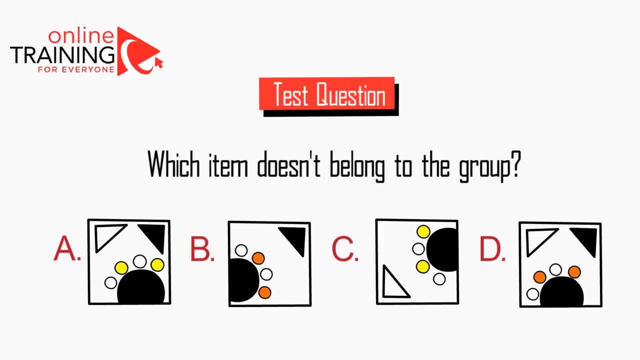 with multiple items. In our choice, we have choices A, B, C and D. Each item is represented as a square which contains multiple different items inside, And you need to determine the item which does not belong to this particular pattern or sequence. Do you see the answer? Please take a. 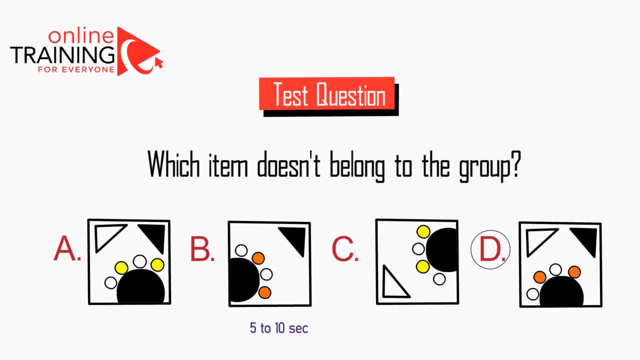 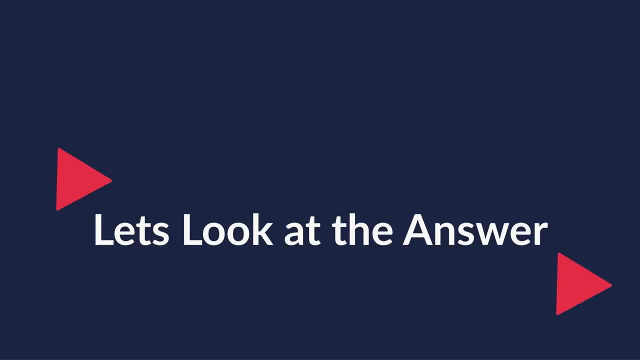 look to see if you can come up with the solution. 5 to 10 seconds, Maybe 10 to 20 seconds to see if you can come up with the answer. Did you figure it out? Let's continue to see how we can go and get to the correct solution together, As you might. 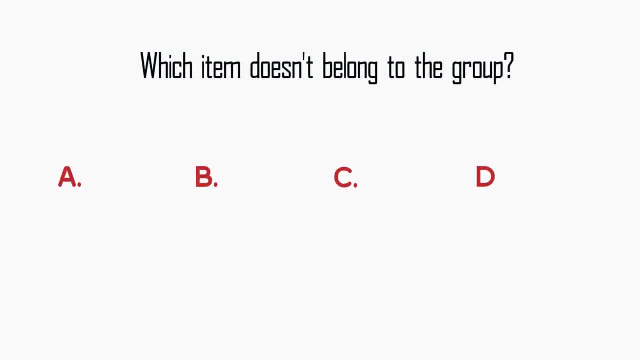 have figured out by now. there is always a pattern that you need to detect to answer these types of questions correctly, And a lot of times there are items that are designed to confuse you. So let me first walk you through the items that are designed to confuse you. You have small circles. 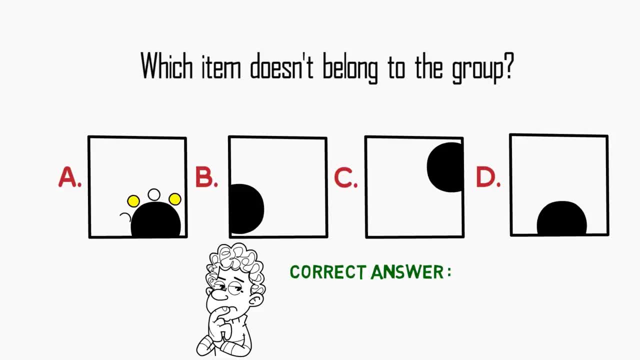 And there are four small circles in each of the square, And the small circles do not have any patterns. We also have triangles. Some squares have two triangles And some squares only have one, But there is no pattern here. The pattern is actually defined by the half circle And, as you 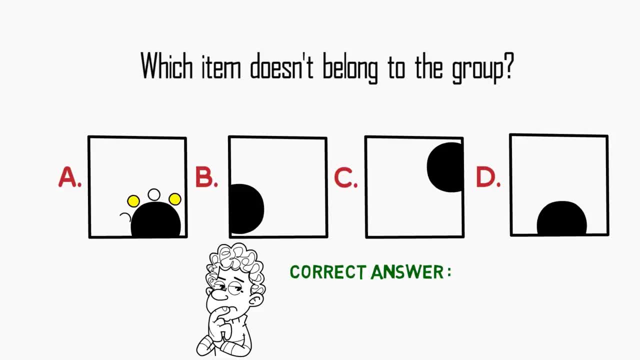 And there are four small circles in each of the square, And the small circles do not have any patterns. We also have triangles. Some squares have two triangles And some squares only have one, But there is no pattern here. The pattern is actually defined by the half circle And, as you 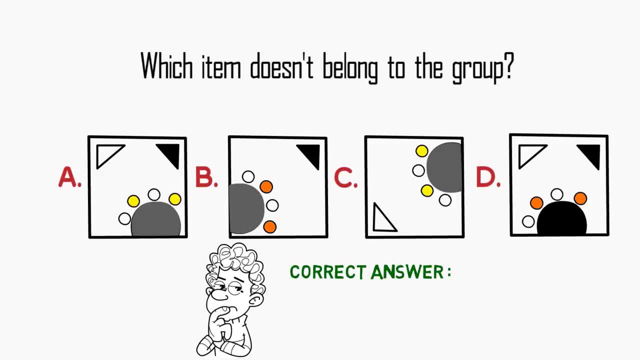 can see, all half circles are attached to the corners of the square. You see this in the shapes A, B and C. But in shape D half circle is placed in a different location. It is in the bottom middle of the square. 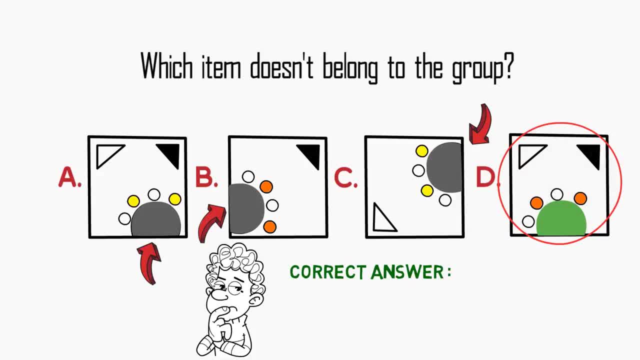 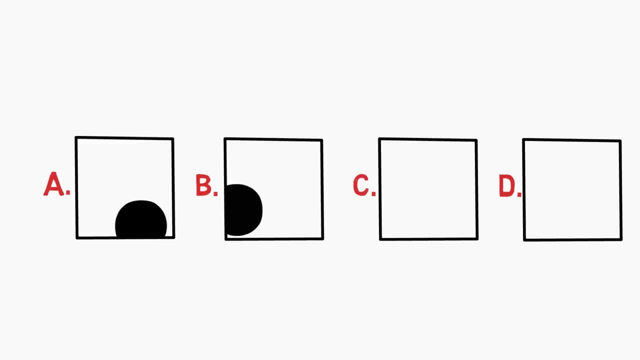 This is why the item that doesn't belong to the group is the choice D. So the correct answer here is choice D. Let's recap: The pattern here is that all half circles are attached to the corners of the square, But half circle in the shape D is placed in a different place than the others. 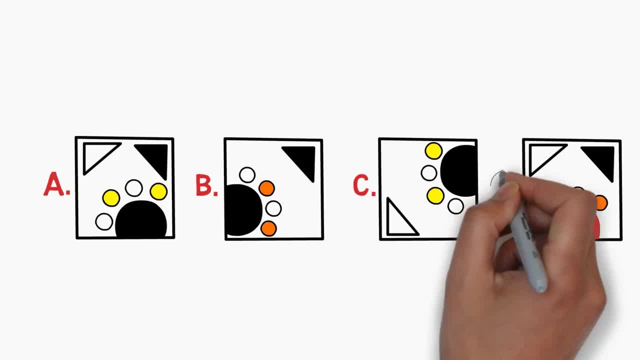 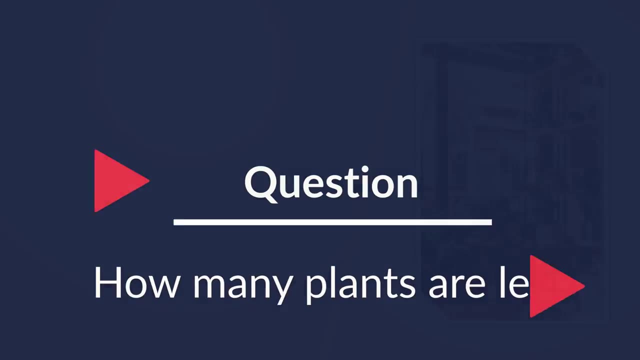 The half circle there is in the lower part of the square. This is why the correct answer here is choice D. Hopefully you've nailed this question and now know how to answer similar problems on the test. Here is the challenging question you might frequently see on the test. 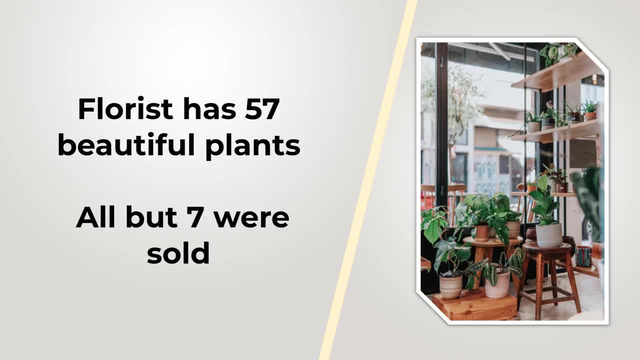 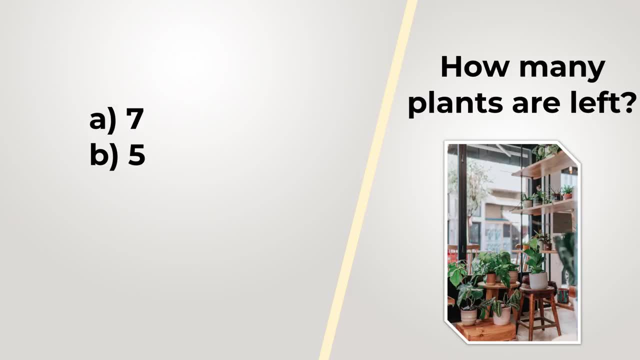 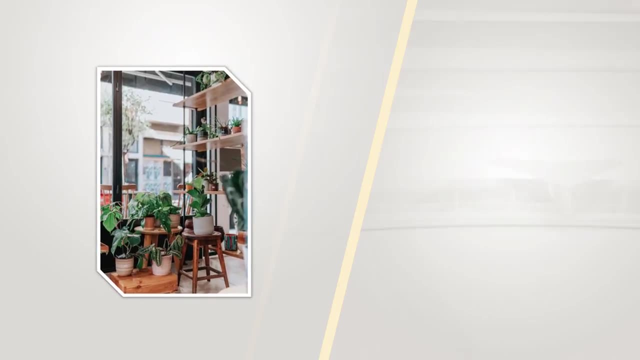 Florist has 57 beautiful plants. All but seven were sold. How many plants are left? There are four different choices: 7,. choice B: 57,, choice C: 64, and choice D: 50.. Take a close look at the solution and see if you might come up with the answer. Give yourself 10 to 15 seconds. This. 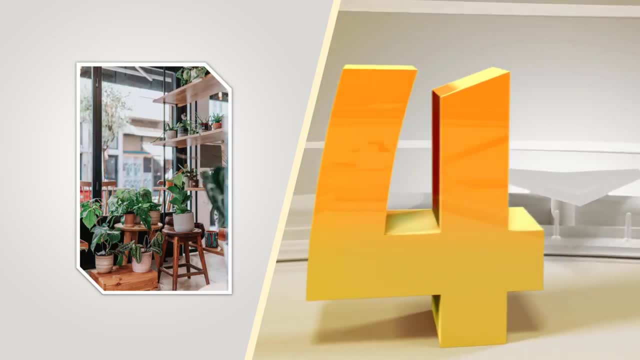 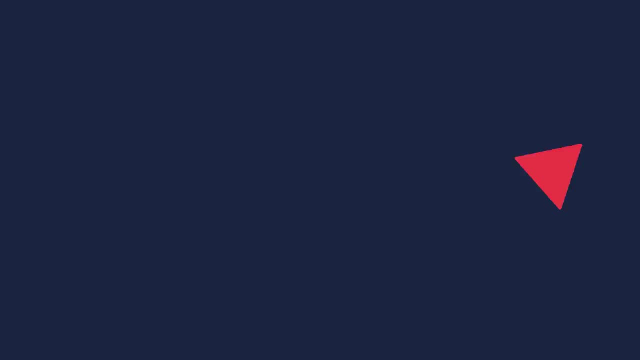 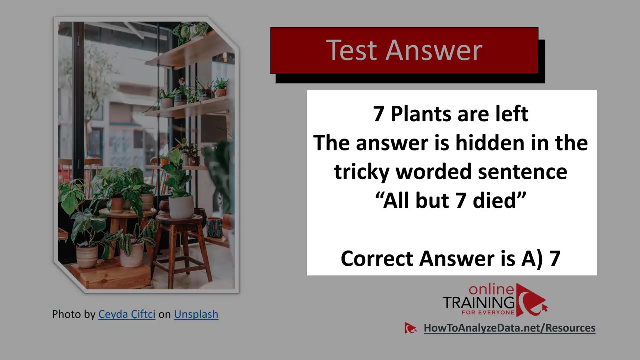 is typically as much time as you would get on the test. Do you think you came up with the answer? Let's continue to see if we can solve this challenge and get to the correct solution together. I think you heard me correctly. So the answer is: 7 plants are left. How is it possible? The answer: 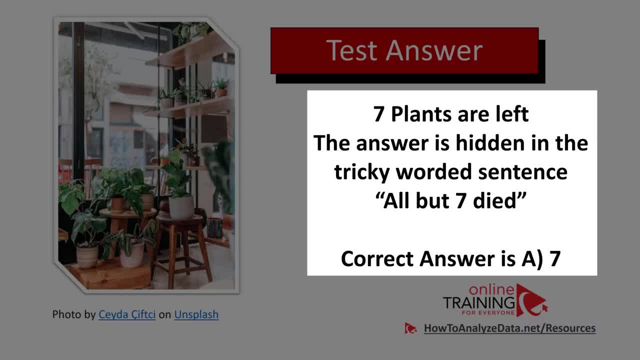 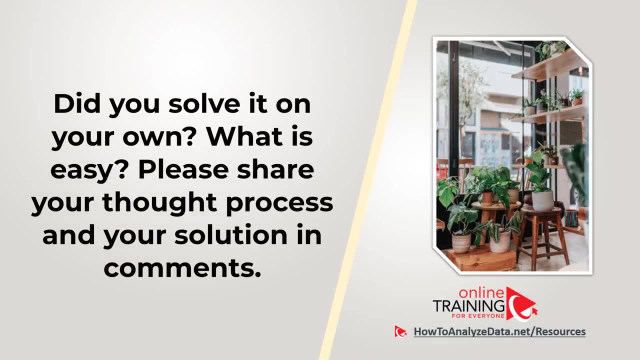 is hidden in the tricky worded sentence: All but seven died. So this is why the correct answer is A. Florist had 57 plants and all of them but seven died. That's why the correct answer is A 7.. Hopefully you've nailed this question and 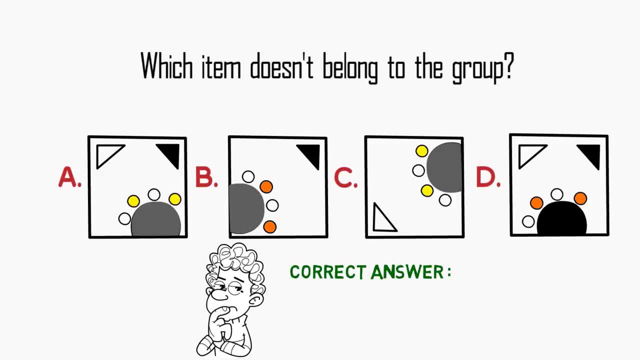 can see, all half circles are attached to the corners of the square. You see this in the shapes A, B and C. But in shape D half circle is placed in a different location. It is in the bottom middle of the square. 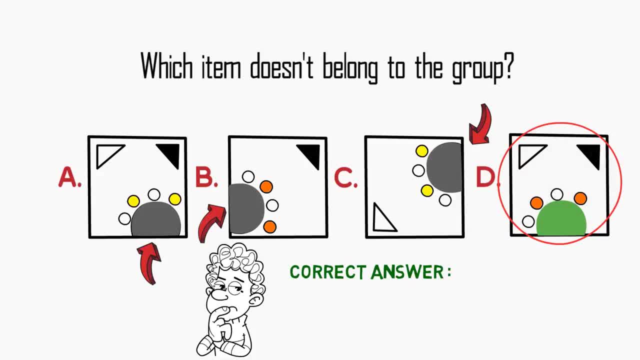 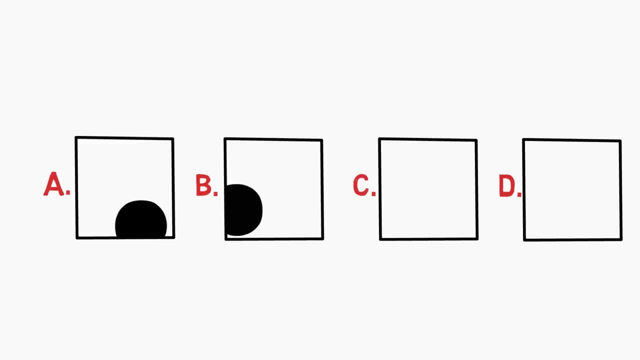 This is why the item that doesn't belong to the group is the choice D. So the correct answer here is choice D. Let's recap: The pattern here is that all half circles are attached to the corners of the square, But half circle in the shape D is placed in a different place than the others. 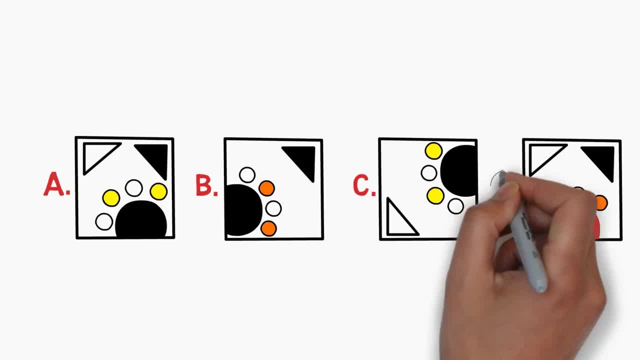 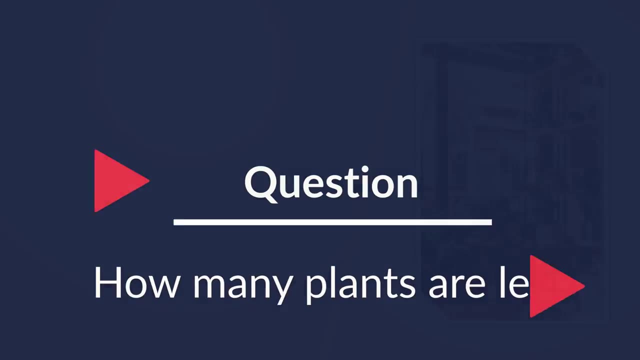 The half circle there is in the lower part of the square. This is why the correct answer here is choice D. Hopefully you've nailed this question and now know how to answer similar problems on the test. Here is the challenging question you might frequently see on the test. 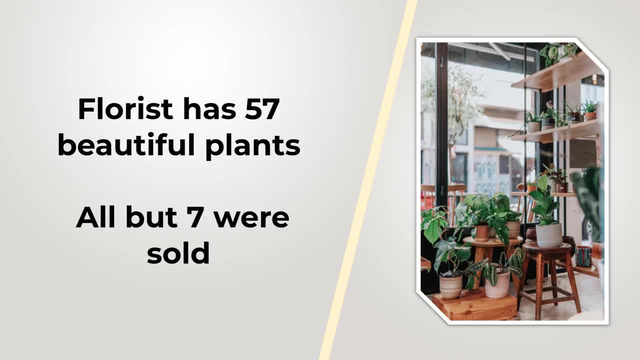 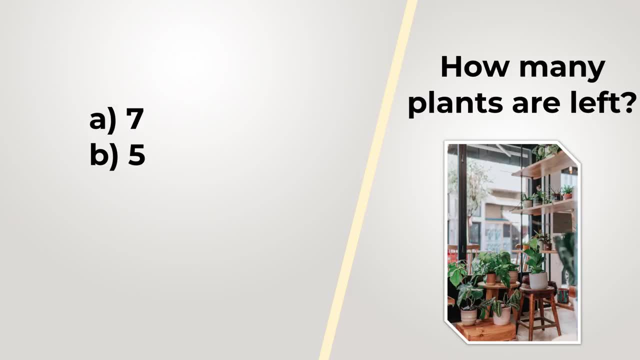 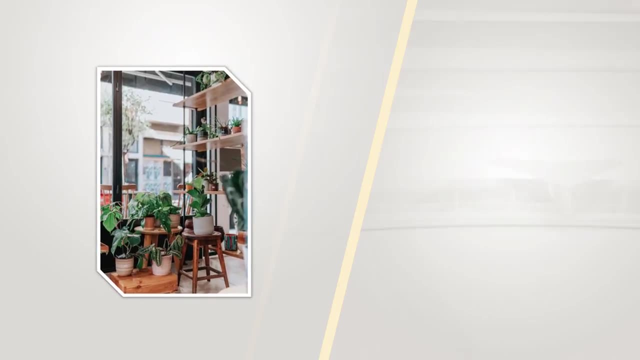 Florist has 57 beautiful plants. All but seven were sold. How many plants are left? There are four different choices: 7,. choice B: 57,, choice C: 64, and choice D: 50.. Take a close look at the solution and see if you might come up with the answer. Give yourself 10 to 15 seconds. This. 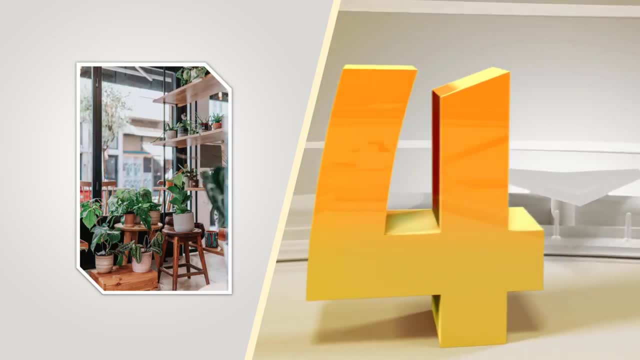 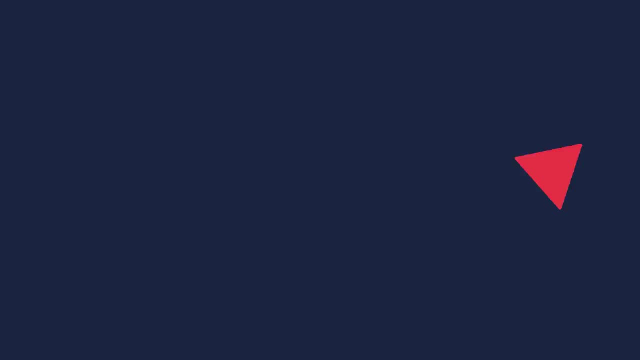 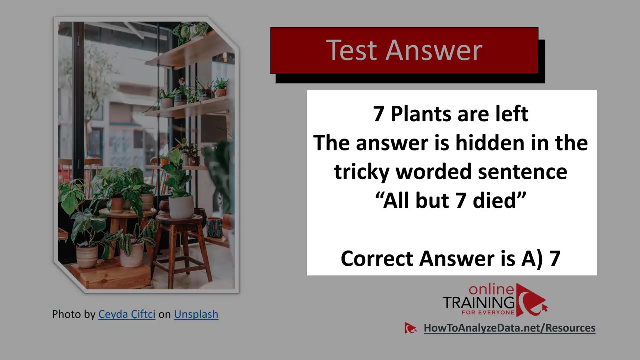 is typically as much time as you would get on the test. Do you think you came up with the answer? Let's continue to see if we can solve this challenge and get to the correct solution together. I think you heard me correctly. So the answer is: 7 plants are left. How is it possible? The answer: 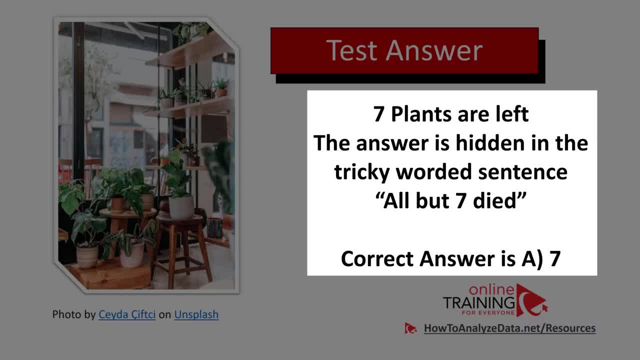 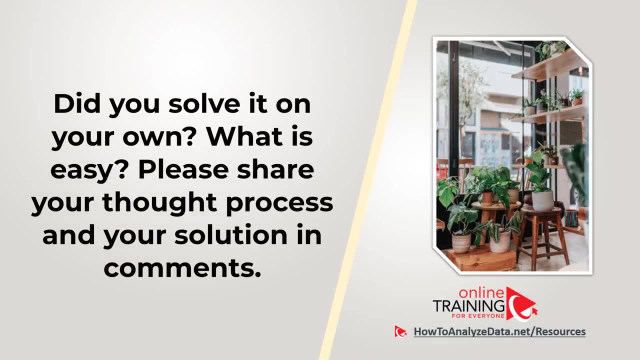 is hidden in the tricky worded sentence: All but seven died. So this is why the correct answer is A. Florist had 57 plants and all of them but seven died. That's why the correct answer is A 7.. Hopefully you've nailed this question and 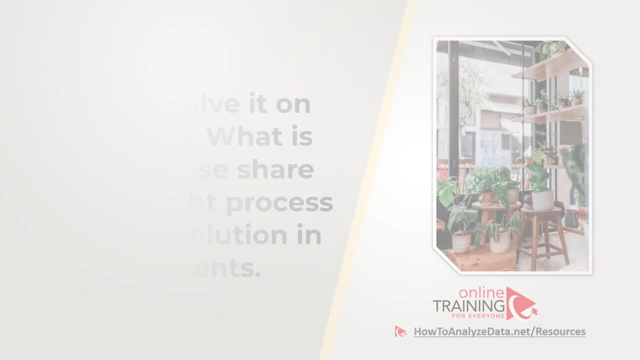 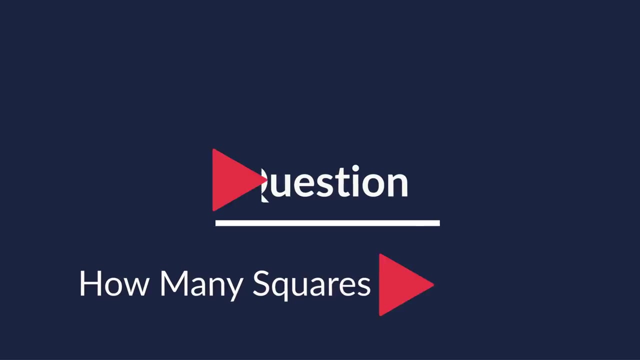 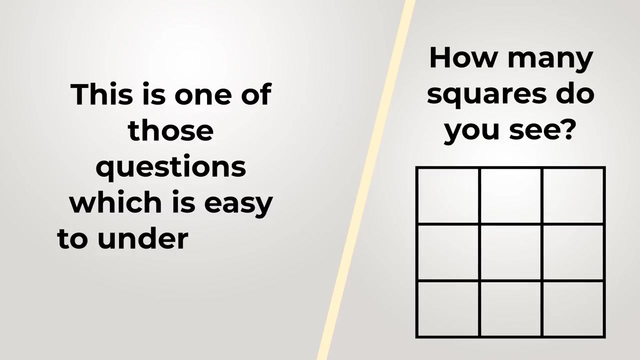 now know how to answer similar problems on the test. I'm very excited to share with you this question, which we frequently see on the test. Despite being tricky, you will have a lot of fun trying to find the answer. This is one of those questions that is easy to understand and it challenges your brain and 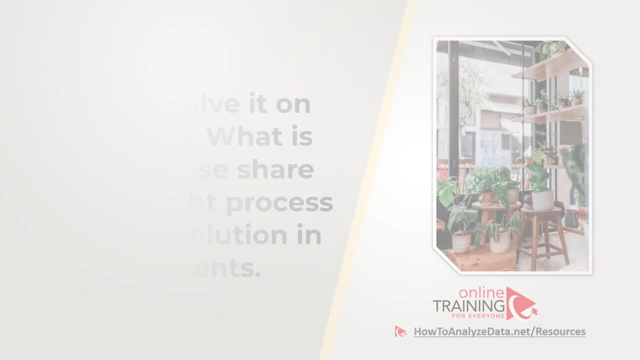 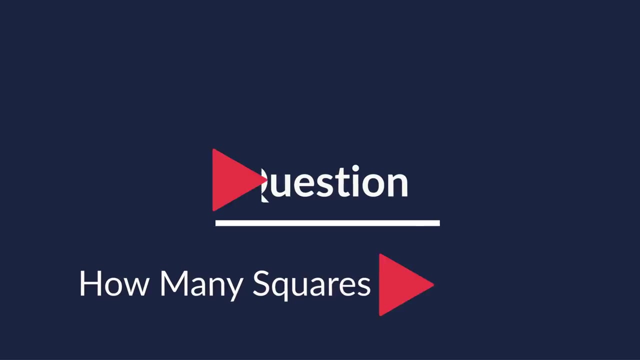 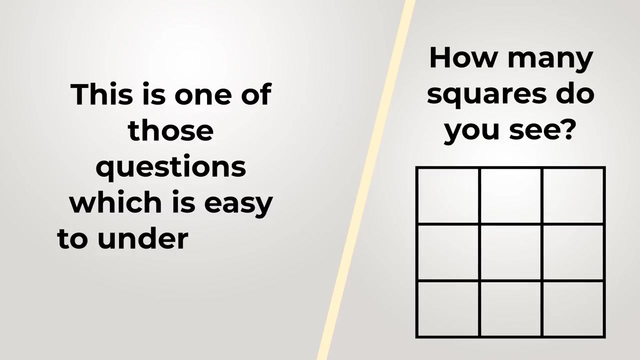 now know how to answer similar problems on the test. I'm very excited to share with you this question, which we frequently see on the test. Despite being tricky, you will have a lot of fun trying to find the answer. This is one of those questions that is easy to understand and it challenges your brain and 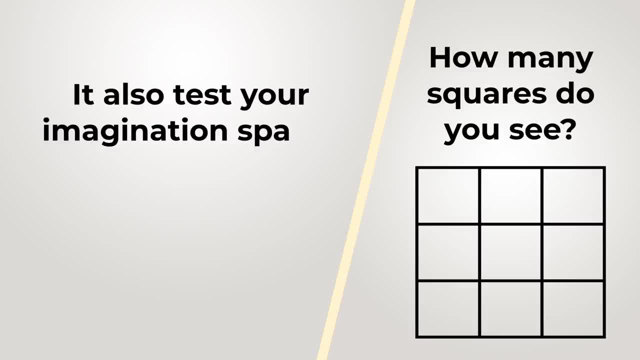 improves your IQ. It also tests your imagination, spatial thinking, logical thinking and attention to details. Take a look at the picture and see how many squares do you see? Think again. The answer might be more challenging than you think. Now might be the good time to pause this video to. 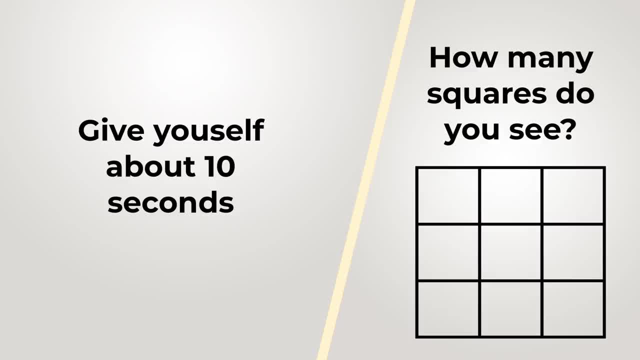 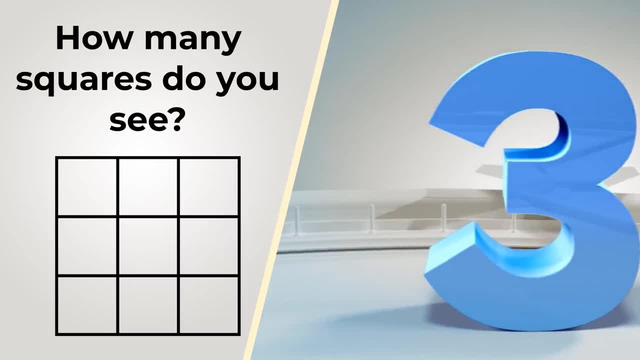 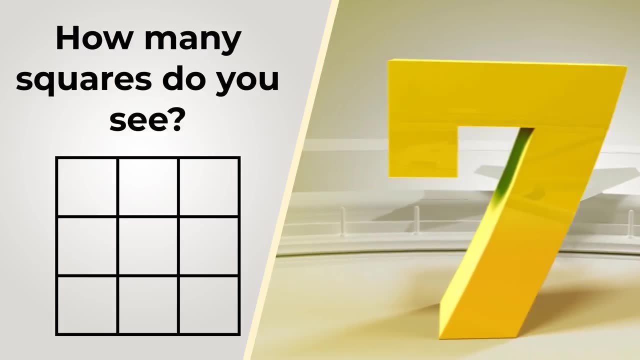 see if you can come up with the answer on your own. Give yourself about 10 seconds. This is typically what you will get on the real test. Do you know the answer? Let me give you a tip. Keep in mind, though, that on a real test, most of the time you don't get any tips, But since we're doing it, 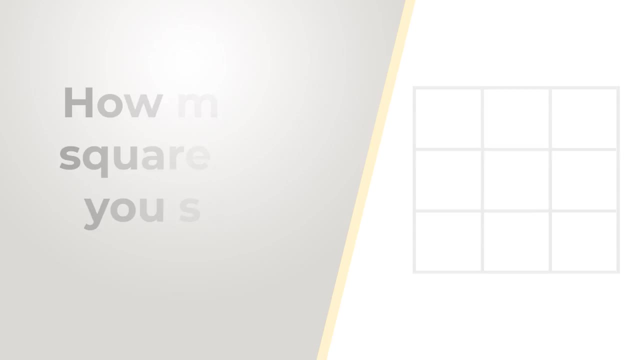 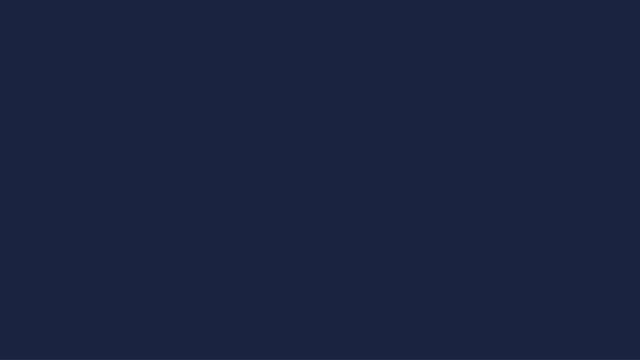 together. I'd like you to consider the possibility of one shape being inside the other. Let's continue to see how we can solve this challenge and get to the correct solution together. There are 18 squares that can be identified in this picture. This definitely came as a big surprise to me. 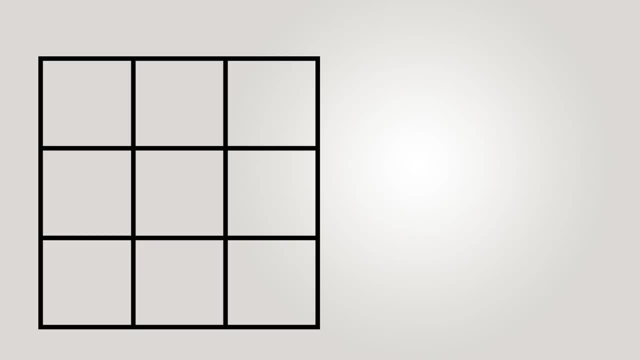 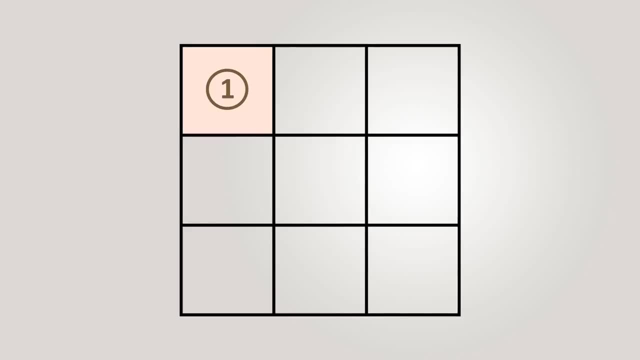 Do you see them all? Some of them might be much easier to identify than others. Let me draw them for you. There are nine small squares: One, two, three, four, five, six, seven, eight, nine. Even those small squares are easy to see and identify. Let's look at the. 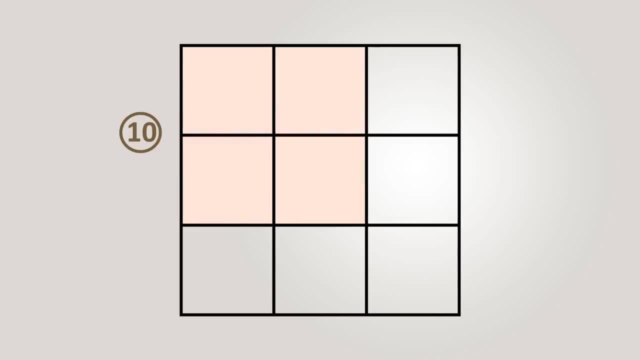 medium-size squares. There are four of them: Number 10., Number 11., Number 12. And number 13.. And then there is one large square. This is number 14.. What do you think about this challenge? Were you able to solve it right away. 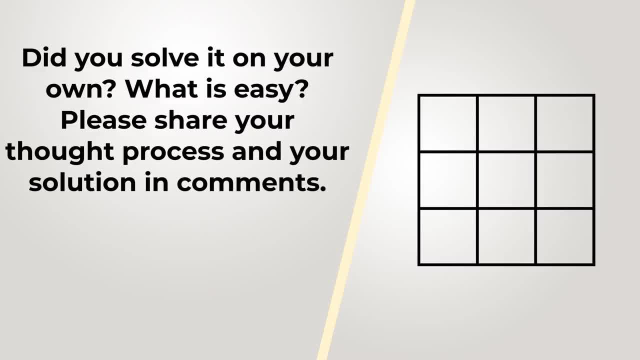 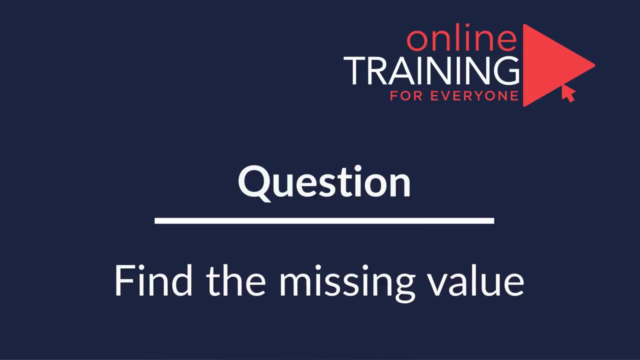 In case you see some additional shapes that we missed, which is always a possibility, please make sure to share them in the comments of this video. Hopefully you've nailed this question and now know how to answer similar problems on the test. I'm extremely excited to share with you the question. 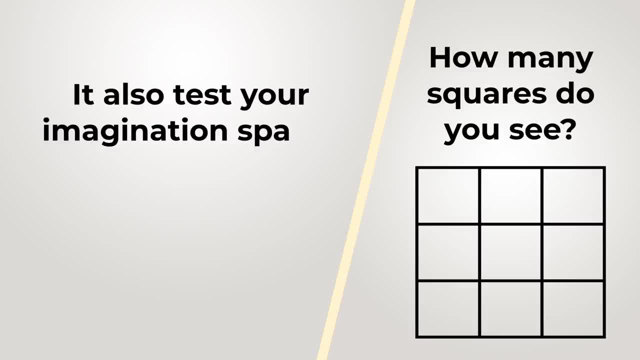 improves your IQ. It also tests your imagination, spatial thinking, logical thinking and attention to details. Take a look at the picture and see how many squares do you see? Think again. The answer might be more challenging than you think. Now might be the good time to pause this video to. 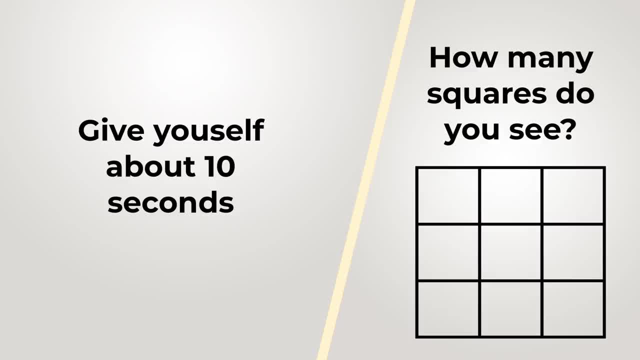 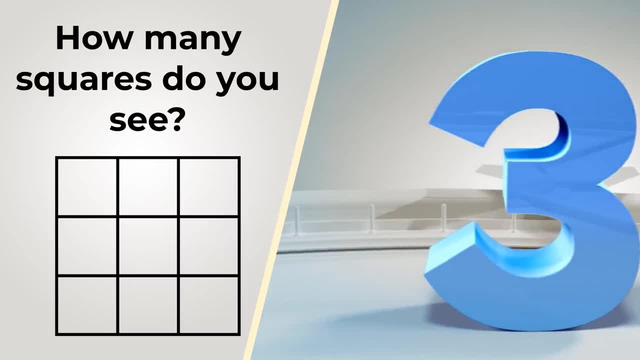 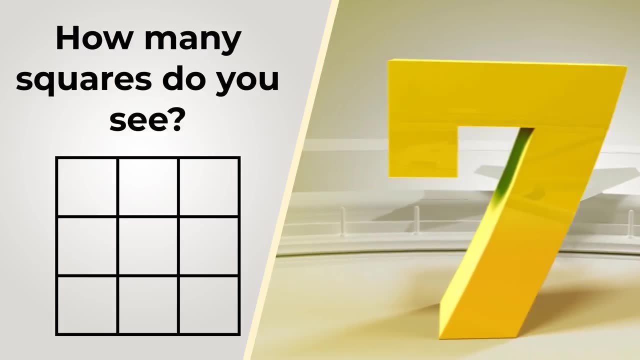 see if you can come up with the answer on your own. Give yourself about 10 seconds. This is typically what you will get on the real test. Do you know the answer? Let me give you a tip. Keep in mind, though, that on a real test, most of the time you don't get any tips, But since we're doing it, 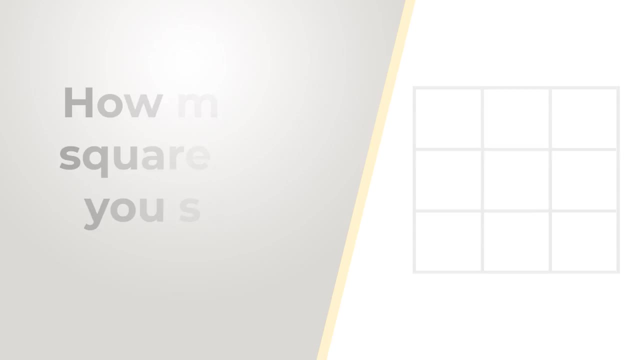 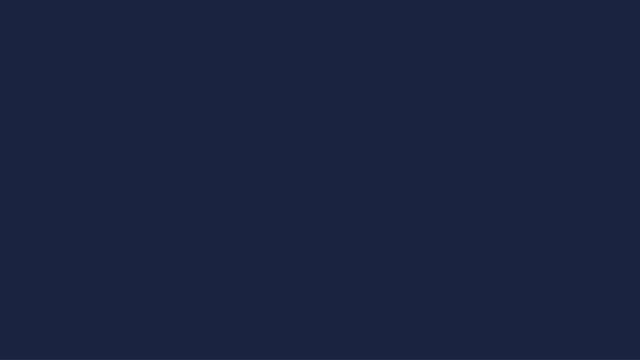 together. I'd like you to consider the possibility of one shape being inside the other. Let's continue to see how we can solve this challenge and get to the correct solution together. There are 18 squares that can be identified in this picture. This definitely came as a big surprise to me. 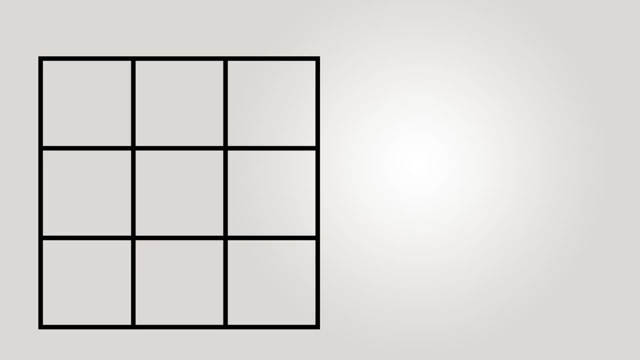 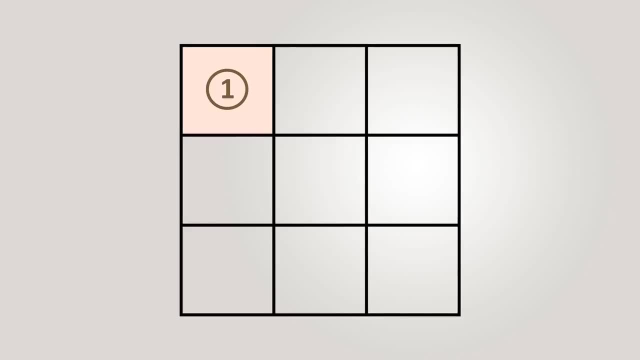 Do you see them all? Some of them might be much easier to identify than others. Let me draw them for you. There are nine small squares: One, two, three, four, five, six, seven, eight and nine. Even those small squares are easy to see and identify. Let's look at the medium-sized. 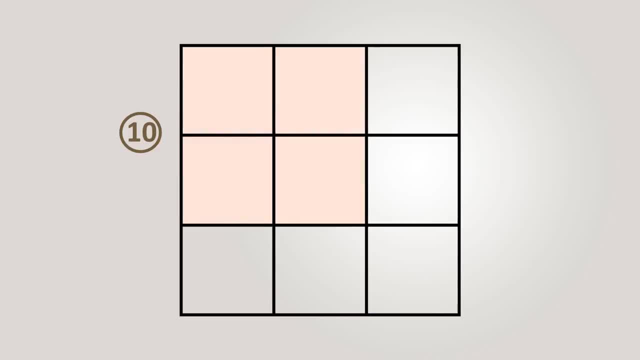 squares. There are four of them: Number 10.. Number 11,, number 12, and number 13.. And then there is one large square. This is number 14.. What do you think about this challenge Were you able to solve? 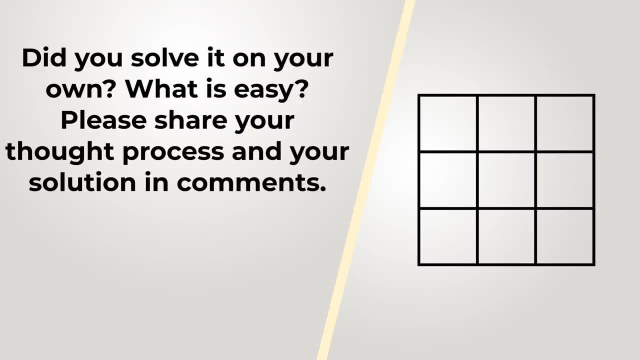 it right away. Please comment below. Thank you for your support. See you in a future video. Bye. In case you see some additional shapes that we missed, which is always a possibility, please make sure to share them in the comments of this video. 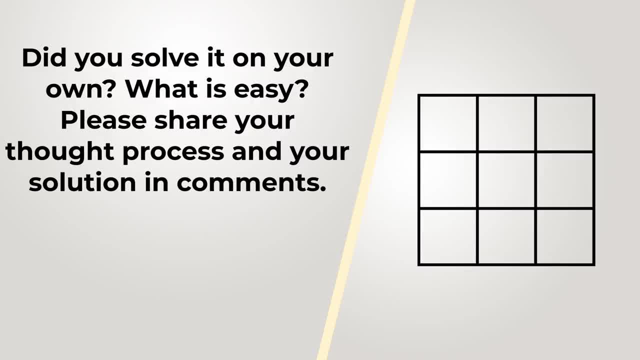 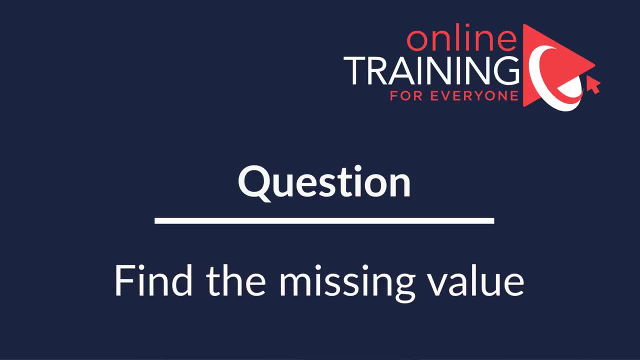 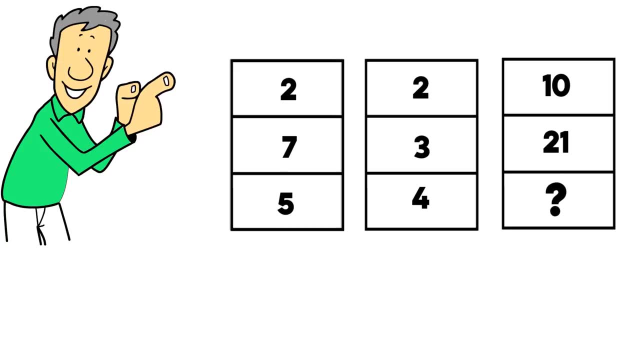 Hopefully you've nailed this question and now know how to answer similar problems on the test. I'm extremely excited to share with you the question that tests your pattern recognition skills. You're presented with three columns. Each column has three numbers. In the first column we see numbers two, seven, five. 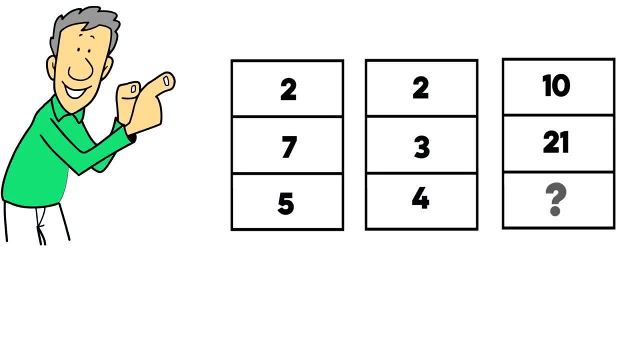 that tests your pattern recognition skills. You're presented with three columns. Each column has three numbers. In the first column we see numbers two, seven, five. In the second, middle column, we see numbers two, three and four. 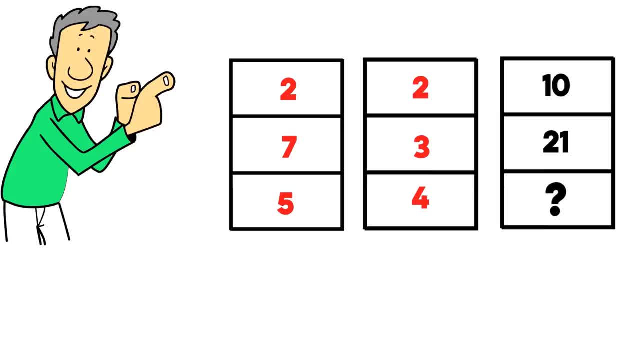 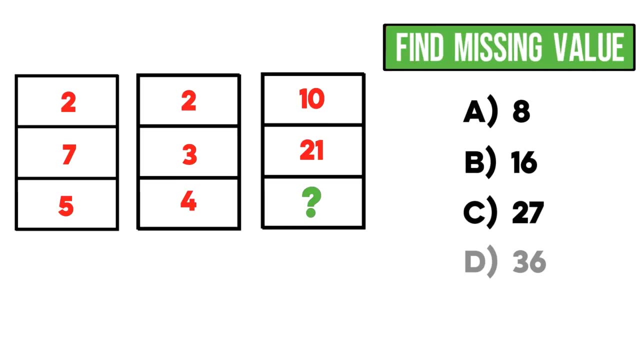 And in the last rightmost column, column number three, we see numbers 10,, 21, and then one number missing. You need to find the missing value, which is highlighted by question mark. You need to find the missing value and you have four choices to choose from. 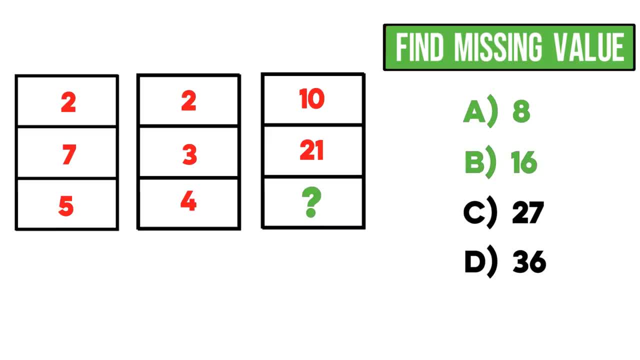 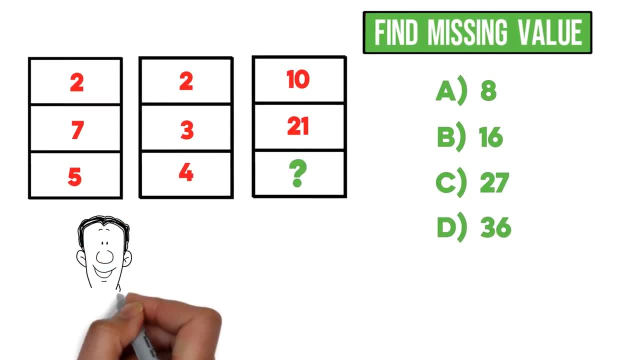 Choice A: eight. Choice B: 16. Choice C: 27. And choice D: 36. Do you think you can recognize missing value? Give yourself five to 10 seconds to see if you can come up with the answer. 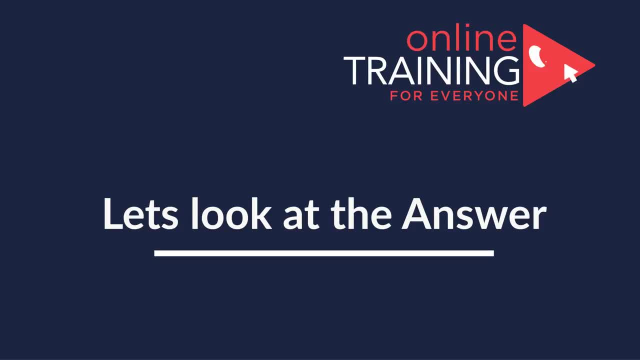 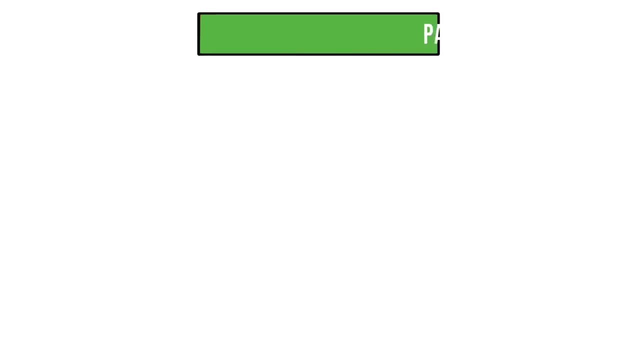 Did you figure out the solution? Let's continue to see how we can get to the correct solution together. The most important skill to solve these types of problems is pattern recognition skill. To recognize the pattern, you need to look closely carefully into each column. 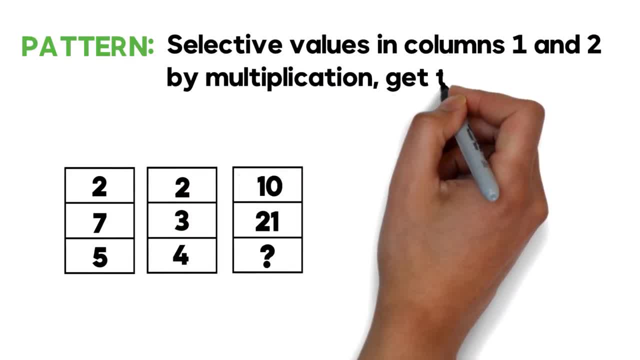 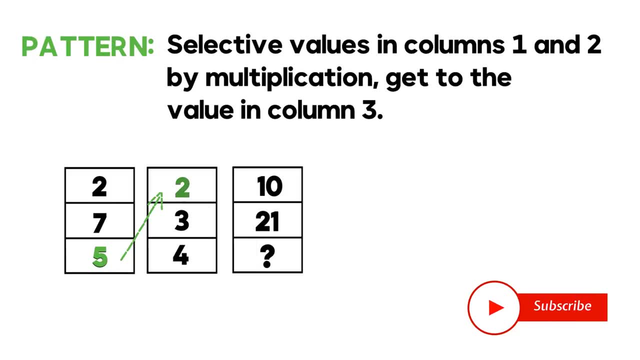 Selective values in columns one and two. by multiplication get to the value in column three, And this is our pattern. Let's take a closer look for the values that are already present. If we multiply five by two, we get to the value of 10.. 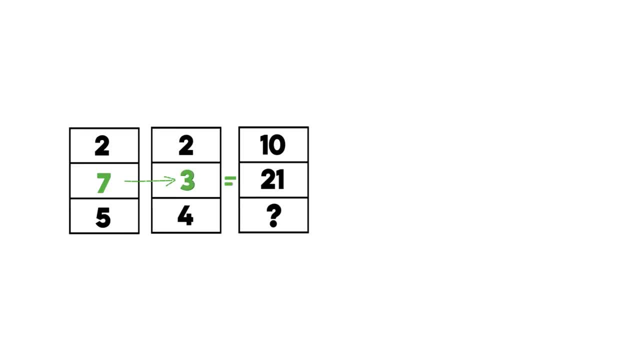 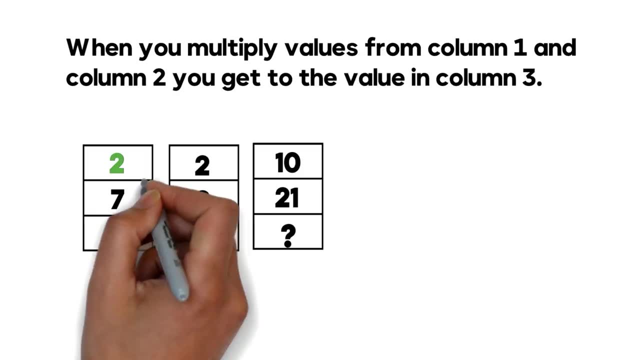 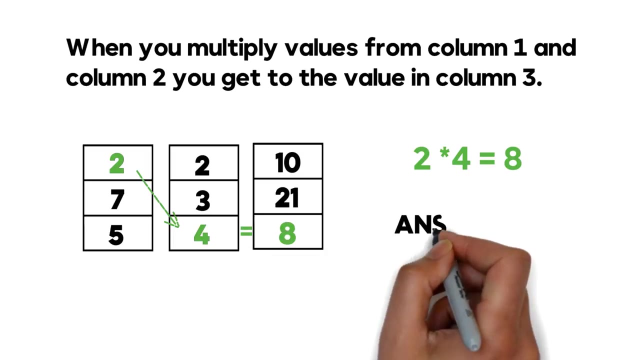 Second set of values, represented by the middle row: seven multiplied by three equals 21.. So the missing values here can be calculated by multiplying two by four, and the end result would be equal to eight. So the correct answer to this problem is choice A, eight. 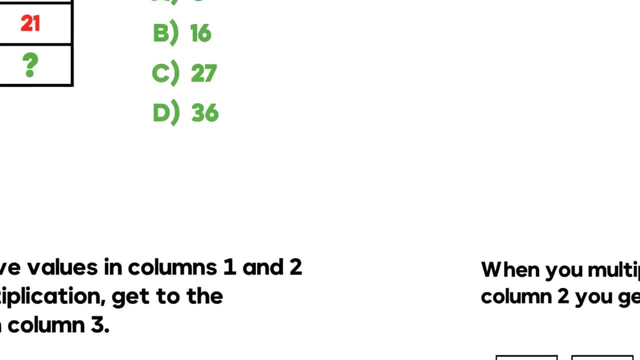 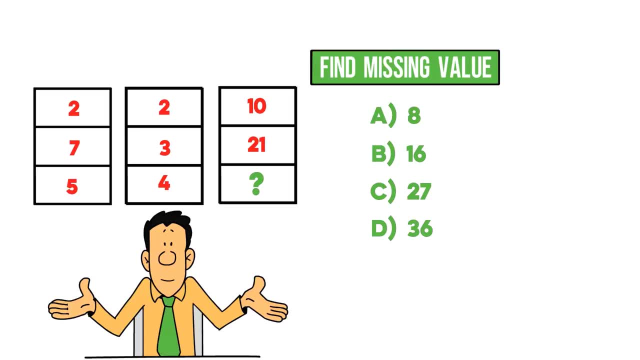 I also wanted to share with you one of the typical mistakes people make as part of answering these types of questions. People start looking at the columns themselves, But unfortunately there's no pattern just by looking in the values in column one, since pattern just doesn't exist. 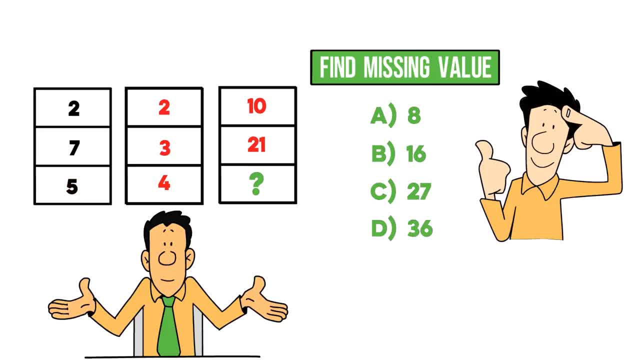 If you look only at the values in column one, or only at the values in column two, or only at the values in column three, you will not be able to come up with the answer. You have to look across and take a global view. 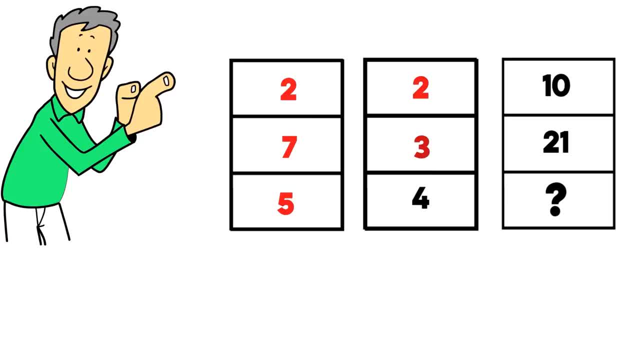 In the second middle column we see numbers two, three and four, And in the last rightmost column, column number three, we see numbers 10,, 21, and then one number missing. You need to find the missing value. 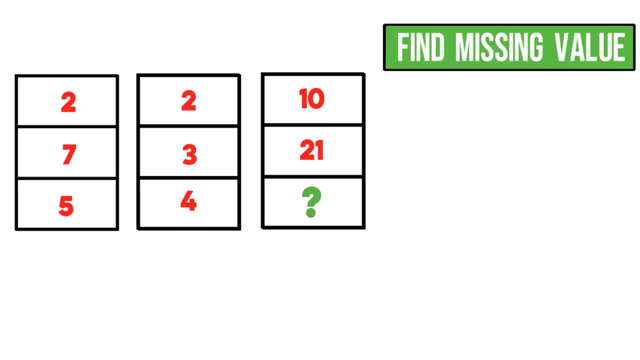 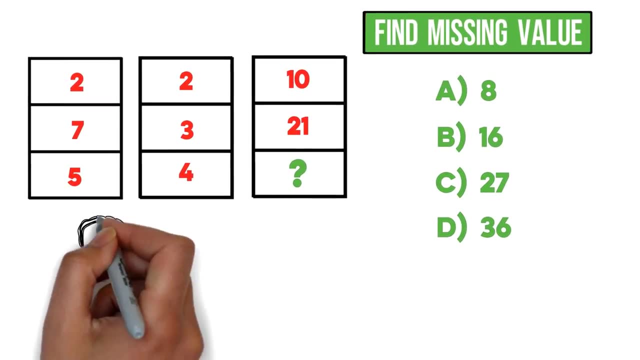 which is highlighted by question mark. You need to find the missing value and you have four choices to choose from: Choice A, eight, Choice B: 16. Choice C: 27. And choice D: 36. Do you think you can recognize missing value? 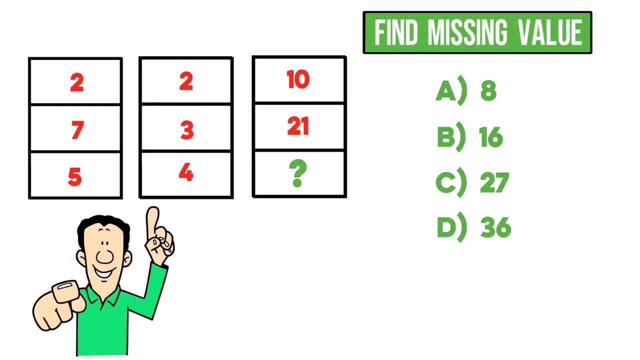 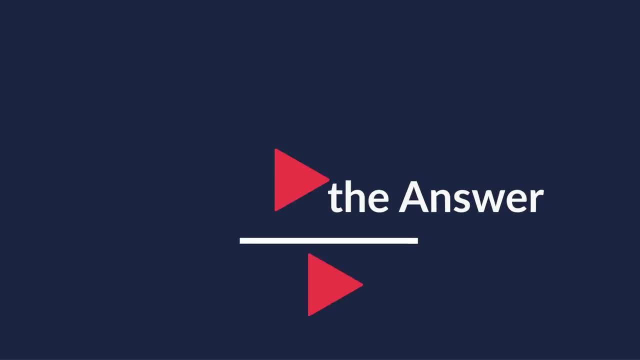 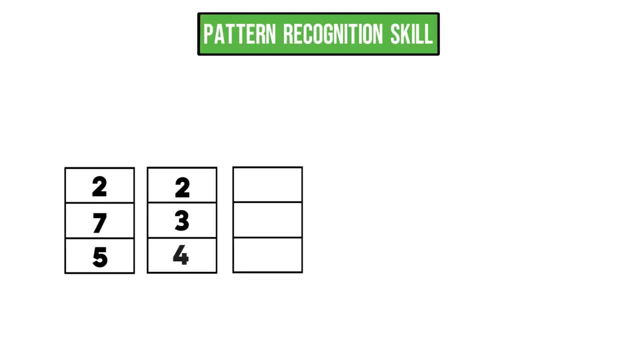 Give yourself five to 10 seconds to see if you can come up with the answer. Did you figure out the solution? Let's continue to see how we can get to the correct solution together. The most important skill to solve these types of problems is pattern recognition skill. 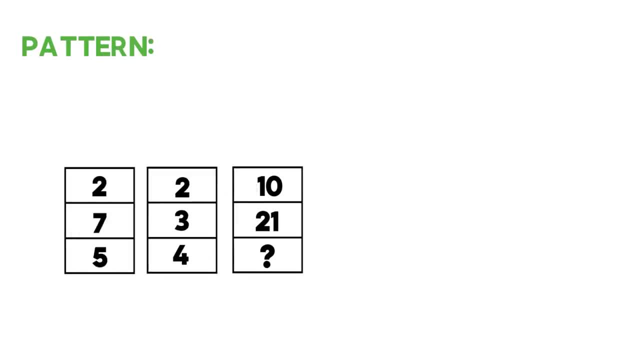 To recognize the pattern, you need to look closely, carefully, into each column. Selective values in columns one and two: by multiplication get to the value in column three, And this is our pattern. Let's take a closer look for the values that are already present. 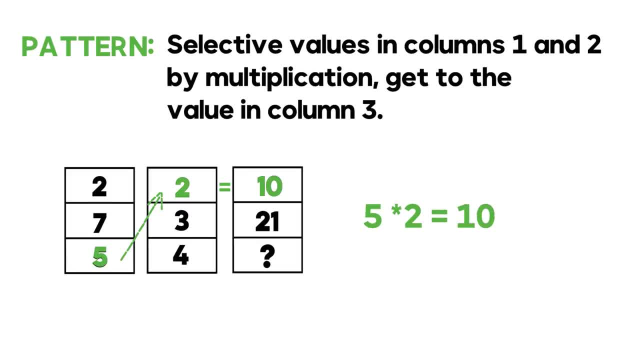 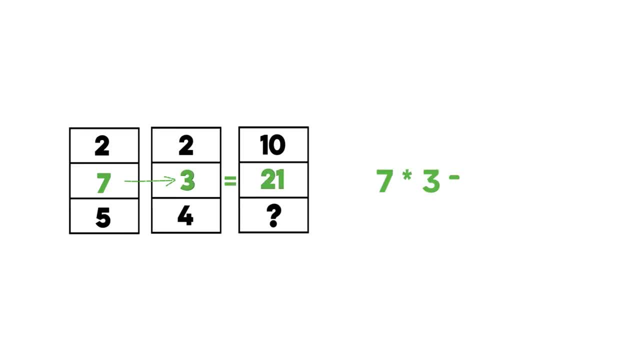 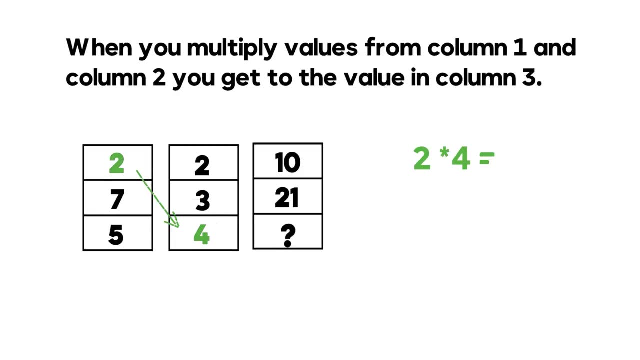 If we multiply five by two, we get to the value of 10.. Second set of values, represented by the middle row: seven multiplied by three equals 21.. So the missing values here can be calculated by multiplying two by four and the end result would be equal to eight. 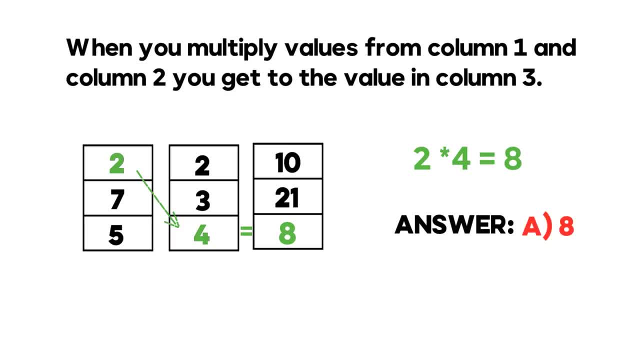 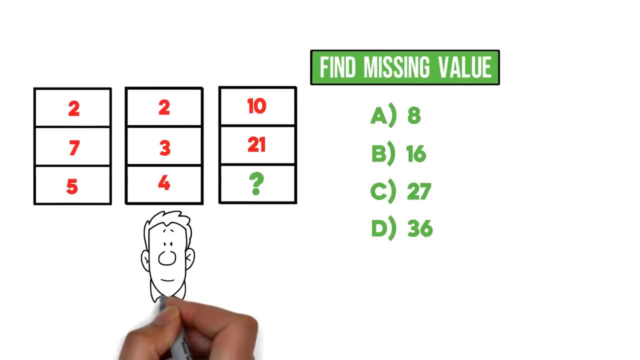 So the correct answer to this problem is choice A eight. I also wanted to share with you one of the typical mistakes people make as part of answering these types of questions. People start looking at the columns themselves, But unfortunately there's no pattern. 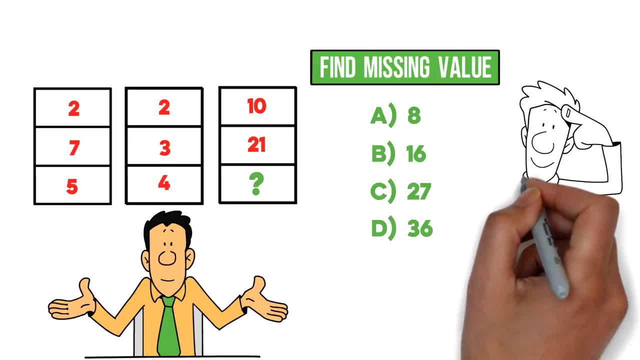 just by looking in the values in column one, since pattern just doesn't exist. If you look only at the values in column one, or only at the values in column two, or only at the values in column three, you will not be able to come up with the answer. 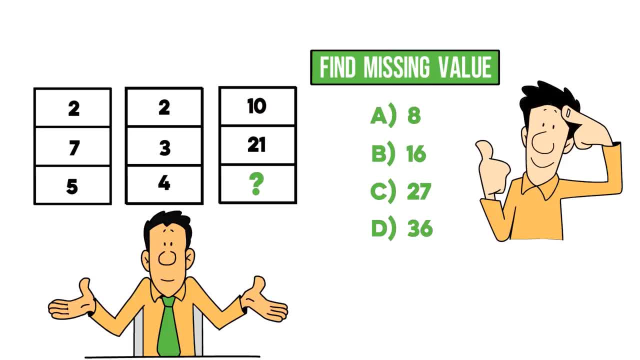 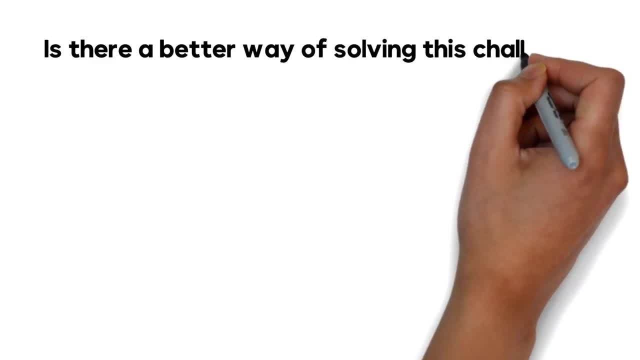 You have to look across and take a global view across multiple columns to get to the correct solution. Can you do me a favor? If you have a better way of solving this challenge, please share your thought process in the comment section of this video. 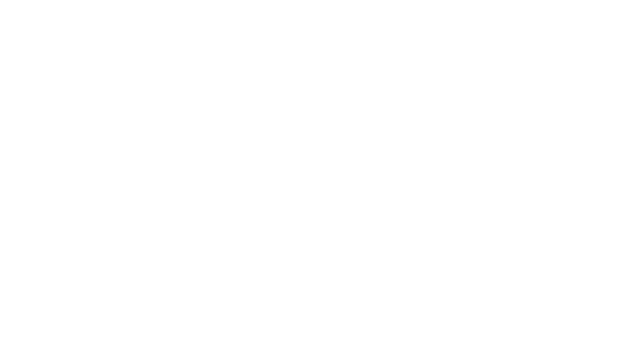 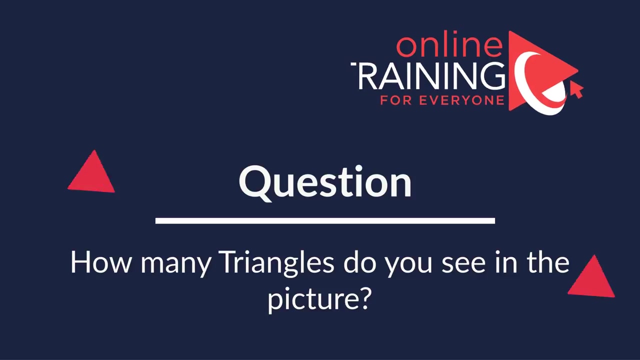 across multiple columns to get to the correct solution. Can you do me a favor? If you have a better way of solving this challenge, please share your thought process in the comment section of this video. This is one of my favorite questions and there is a very high chance that you will get it. on assessment: 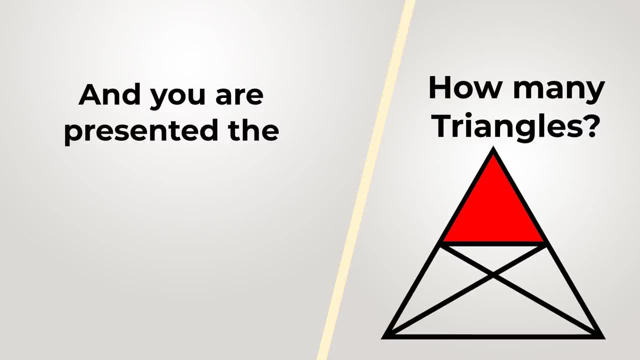 test. How many triangles do you see? You're presented with the shape. on the left There are large triangles and there are also lines inside of these large triangles. You have four different choices: Choice A: 9 triangles. Choice B: 12.. Choice C: 17. And choice D: 24. One triangle. 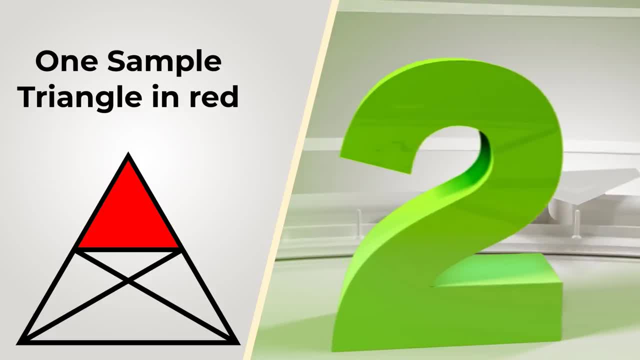 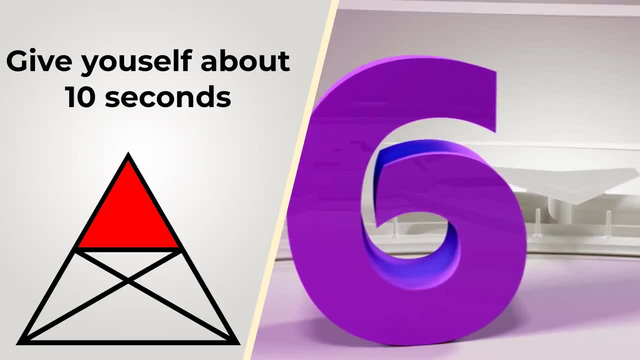 is highlighted in red, but there are a lot of other triangles. Do you think you know the answer? Give yourself a few seconds. I would recommend 10 to 15 seconds. This is about as much time as you will get in the real test. You can pause this video to give yourself some time to figure out the 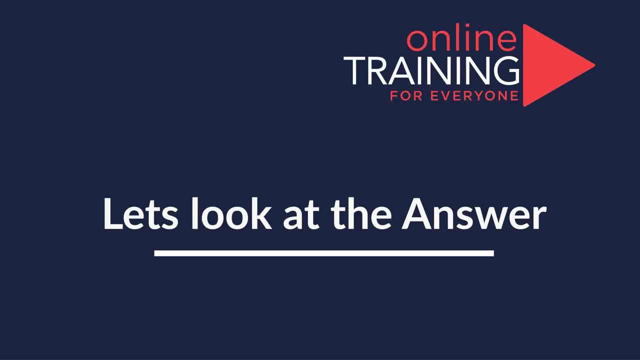 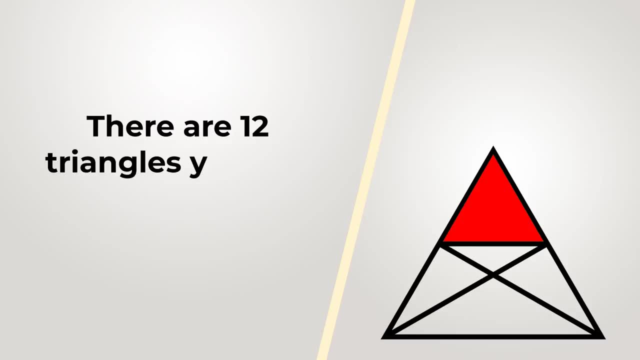 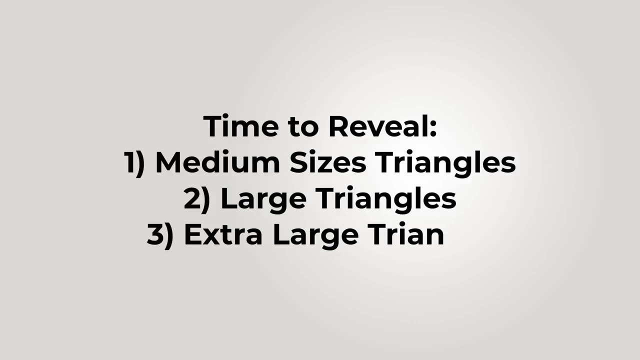 answer. I'm going to continue and reveal the correct solution so we can get to the answer together. I counted 12 triangles in this picture. Is this what you got too? Let me show them all for you. I'll start with the smaller triangles and then go to the medium-sized ones. 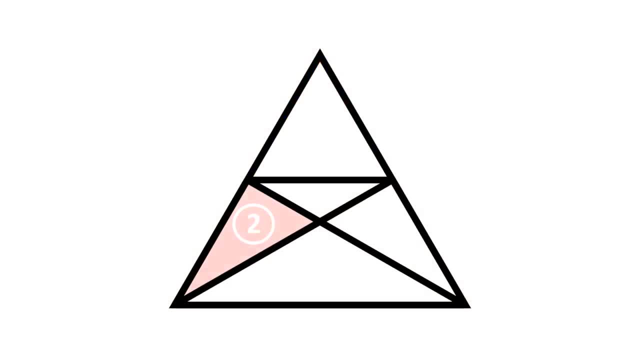 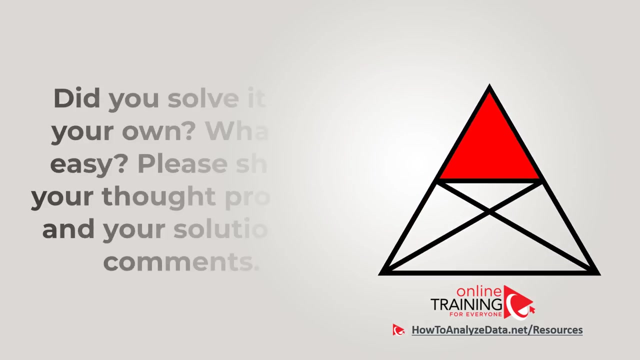 and then go to the large ones: 1,, 2,, 3,, 4,, 5,, 6,, 7,, 8,, 9,, 10,, 11, and 12.. Did you come up with the different answer? Please share your thought process in the comment section of this video. 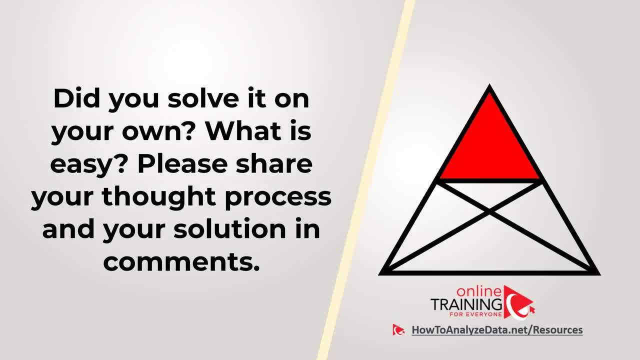 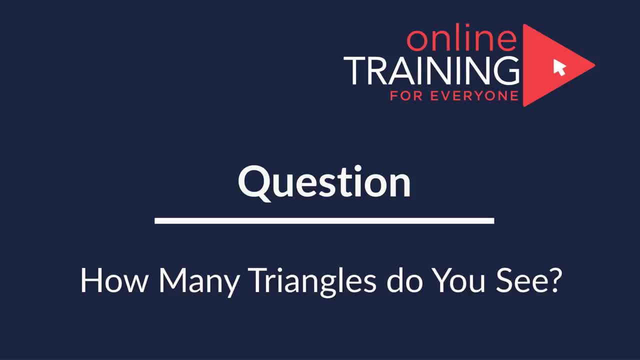 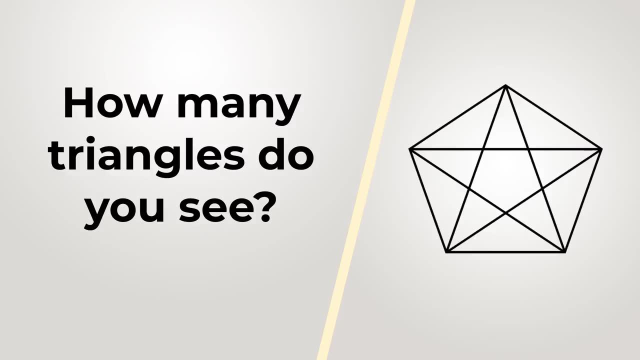 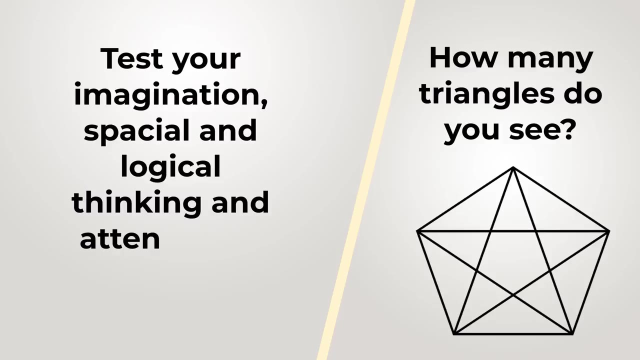 so we can all learn from your practice. Here is the very interesting question from the real test some of you might find challenging. Despite being tricky, you will have a lot of fun trying to find the solution Because this question tests your imagination, spatial thinking, logical thinking and attention. 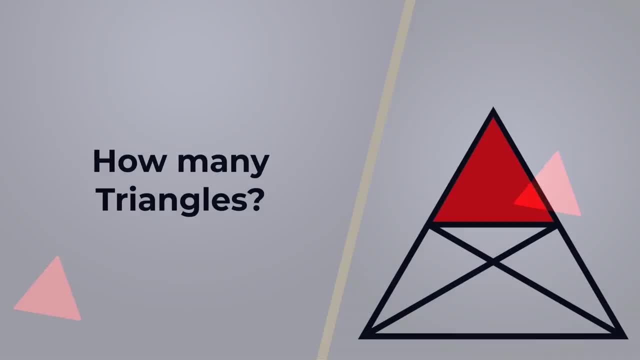 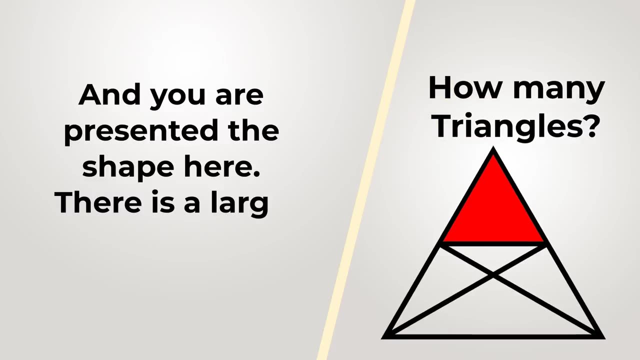 This is one of my favorite questions and there is a very high chance that you will get it on assessment test. How many triangles do you see? You're presented with the shape on the left. There are large triangles and there are also lines inside of these large triangles. You have four. 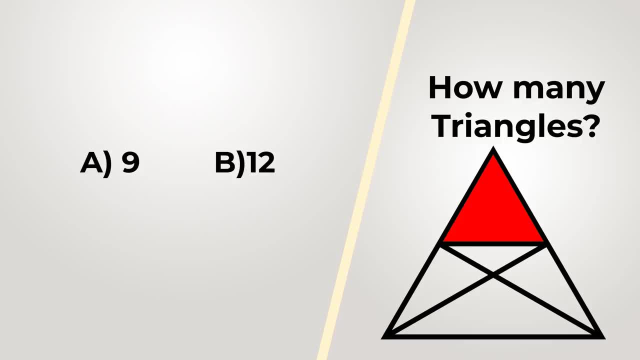 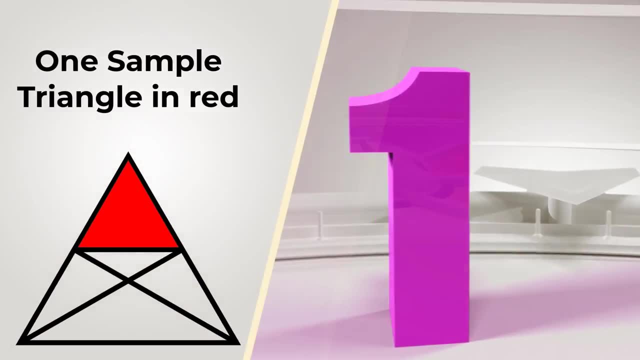 different choices: Choice A: 9 triangles. Choice B: 12. Choice C: 17. And choice D: 24. One triangle is highlighted in red, but there are a lot of other triangles. Do you think you know the answer? 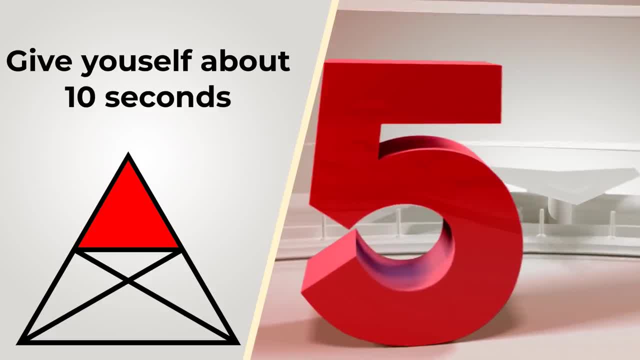 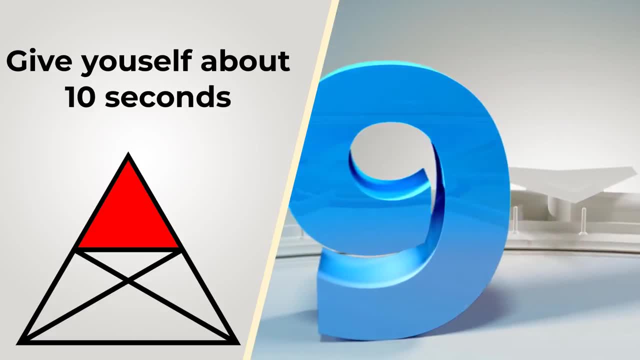 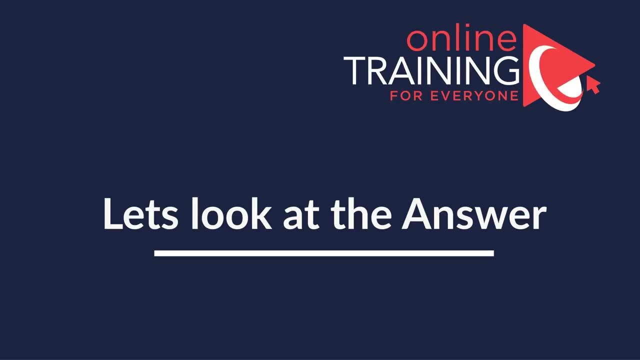 Give yourself a few seconds. I would recommend 10 to 15 seconds. This is about as much time as you will get in the real test. You can pause this video to give yourself some time to figure out the answer. I'm going to continue and reveal the correct solution so we can get to the answer. 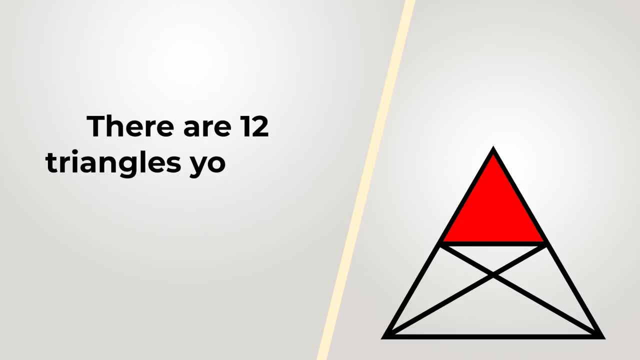 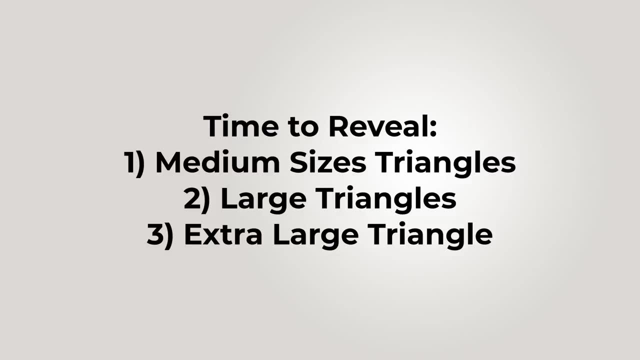 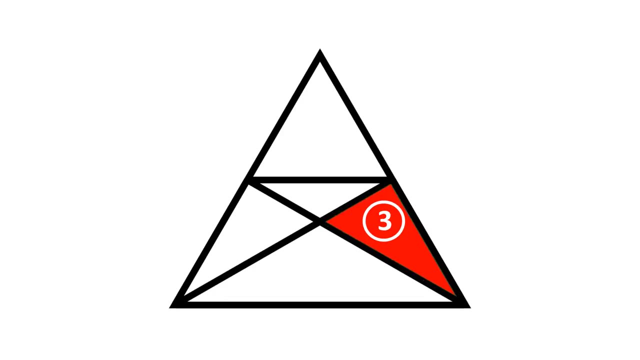 together. I counted 12 triangles in this picture. Is this what you got too? Let me show them all for you. I'll start with the smaller triangles and then go to the medium-sized ones and then go to the large ones: 1,, 2,, 3,, 4,, 5,, 6,, 7,, 8,, 9,, 10,, 11, and 12.. Did you come up with? 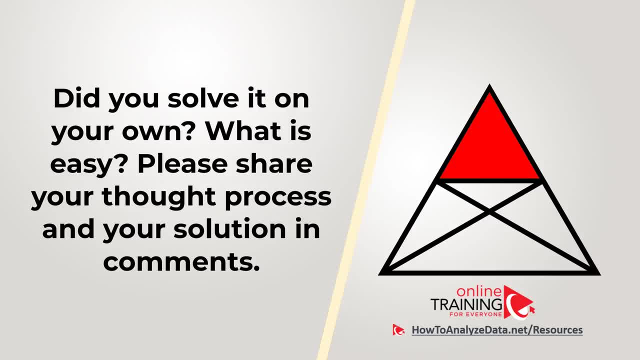 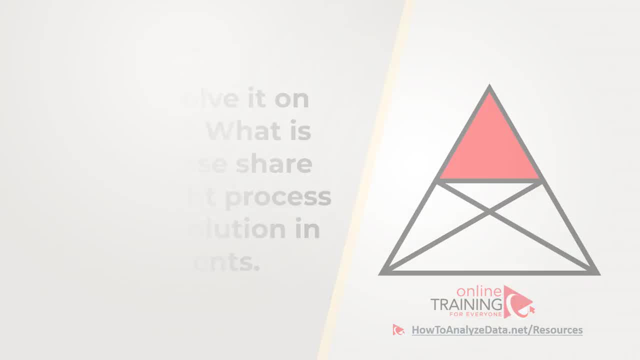 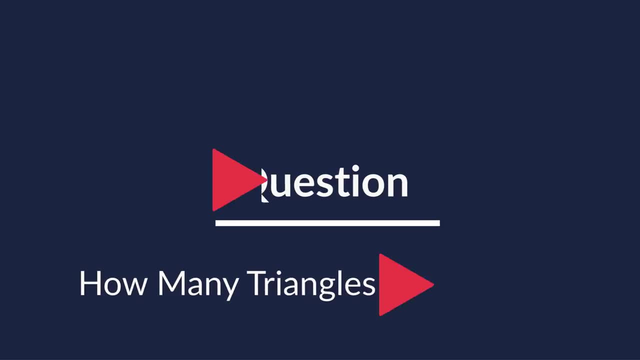 the different answer. Please share your thought process in the comment section of this video so we can all learn from your practice. Here is the very interesting question from the real test some of you might find challenging. Despite being tricky, you will have a lot of fun trying to find the solution. 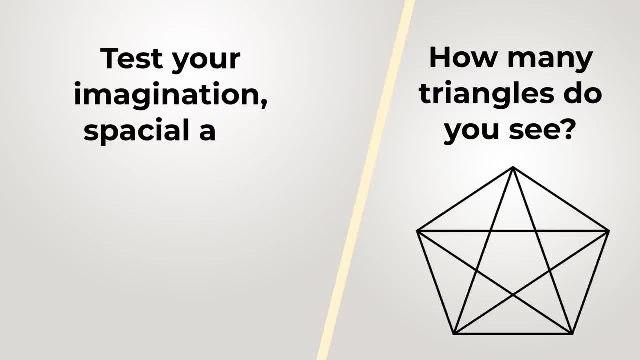 Because this question tests your imagination, spatial thinking, logical thinking and attention to details. Please take a look at the picture and identify all triangles in this picture. Do you think you know the answer? Now might be the right time to pause this video to see if you can. 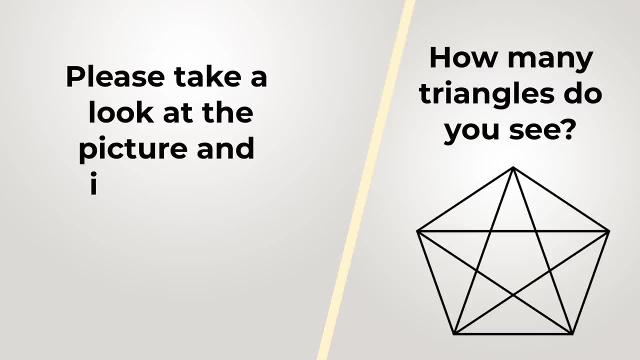 to details. Please take a look at the picture and identify all triangles in this picture. Do you think you know the answer? Now might be the right time to pause this video to see if you can come up with the answer on your own. Give yourself about 10 seconds. This is typically about as much. 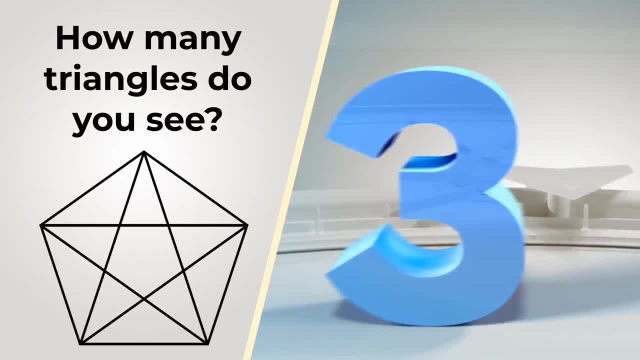 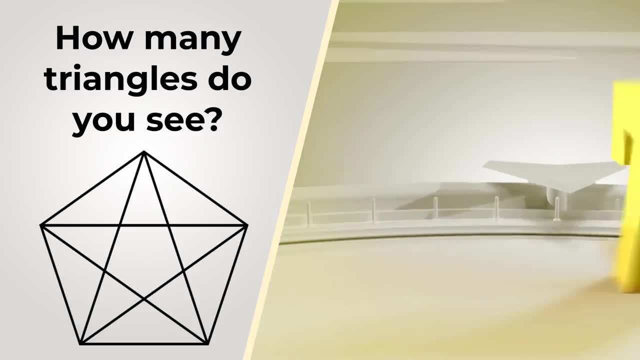 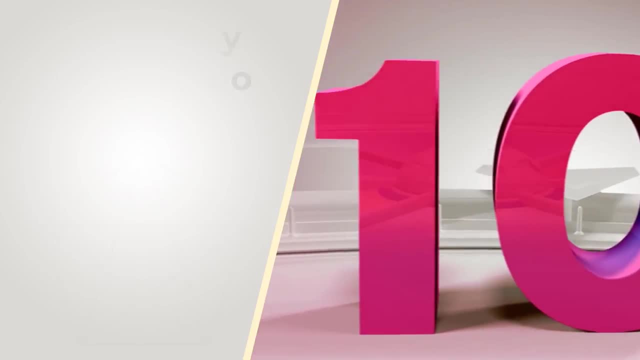 time you will get. on the real test, Did you come up with the answer? Let me give you a tip. Keep in mind, though, that on the real test, nobody is going to give you any suggestions, But make sure to consider the possibility of one shape being inside the other. Now let's continue to see if we 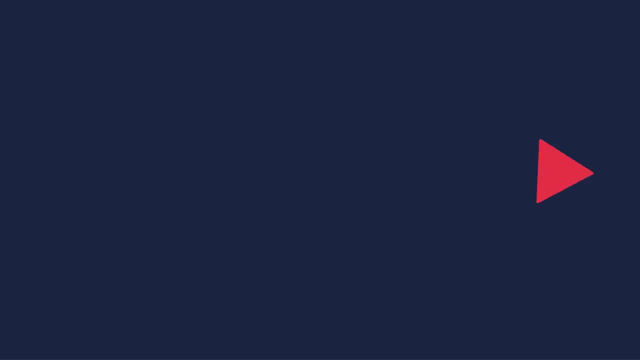 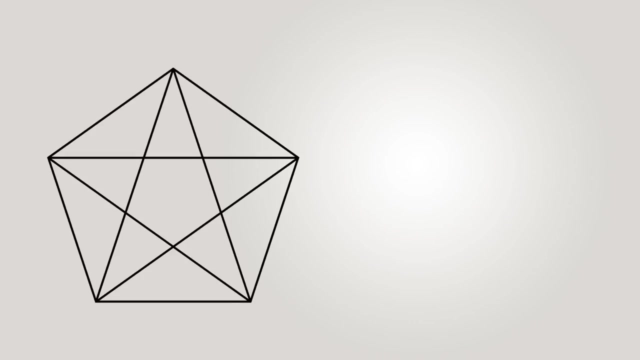 can solve this challenge and get to the correct solution together. It is mind-boggling, but there are 35 triangles here. Can you believe? it Certainly was a huge surprise to me as I was discovering them. Let me draw all of them for you. I will start by drawing small border triangles. 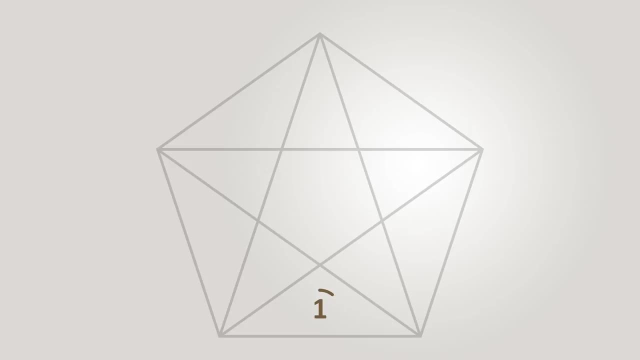 There are 10 of them. Please count with me: 1,, 2,, 3,, 4,, 5,, 6,, 7,, 8,, 9, and 10.. Now let's do next 10 triangles: 11,, 12,, 13,, 14,, 15,, 16,, 17,, 18,, 19,, 20,, 21,, 22,, 23,, 24,, 25,, 26,, 27,, 28,, 29,, 30,. 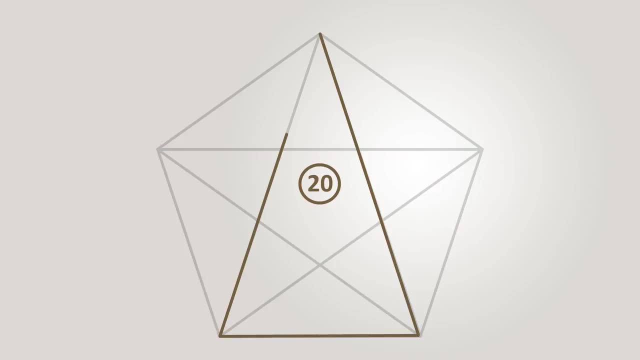 21,, 22,, 23,, 24,, 25,, 26.. And now let's do the next: 5. 21,, 22,, 23,, 24,, 25.. Another 5. 26,, 27,, 28,, 29,, 30 and then the last 5. 31,. 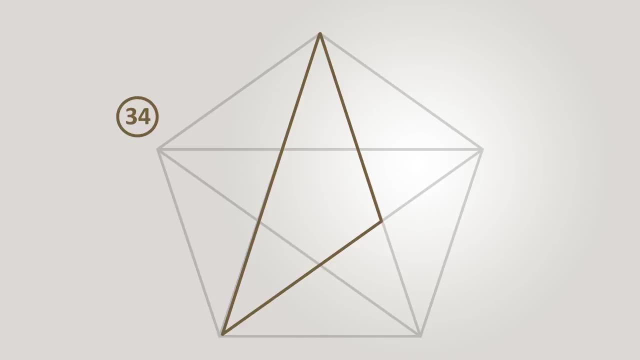 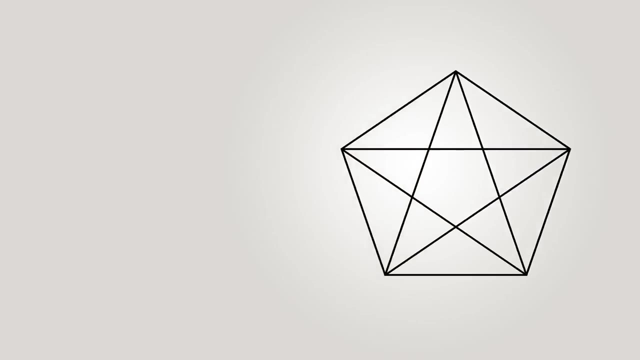 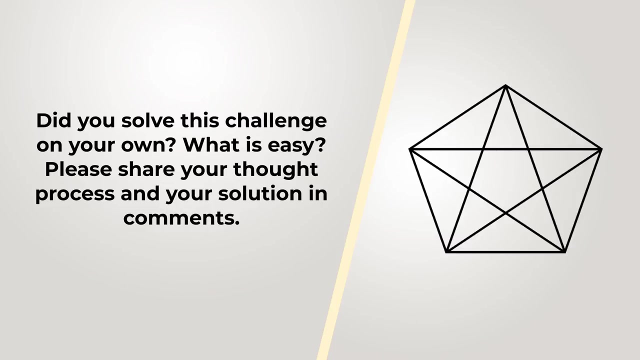 32, 33, 34 and the last one is 35.. do you think we missed any? please make sure to leave your comment and let us know if there is even more. hopefully you nailed this question and now learn how to answer similar questions on the test. 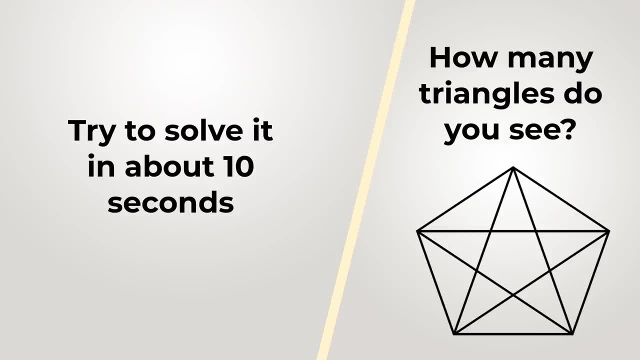 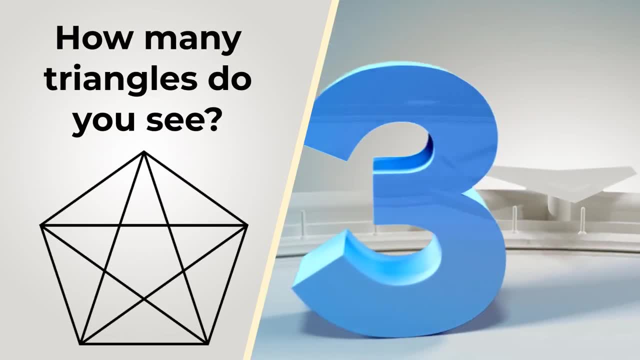 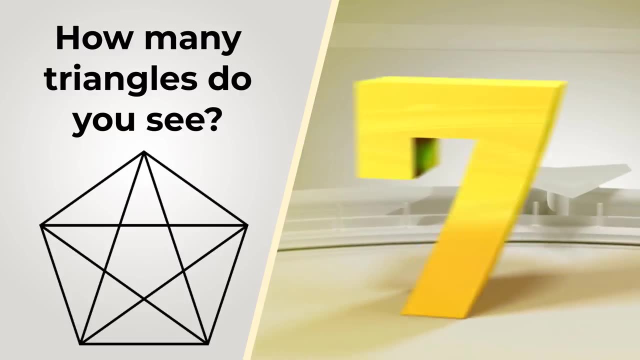 come up with the answer on your own. Give yourself about 10 seconds. This is typically about as much time you will get on the real test. Did you come up with the answer? Let me give you a tip. Keep in mind, though, that on the real test, nobody is going to give you any suggestions, But make sure. 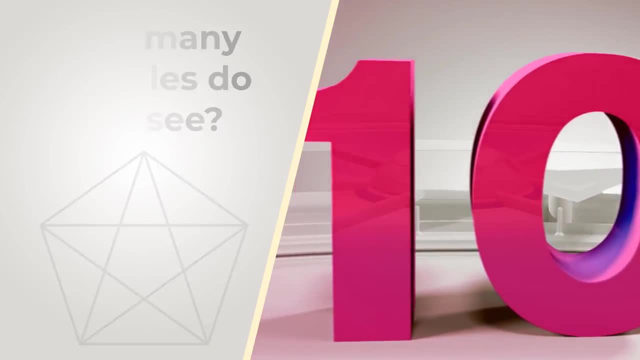 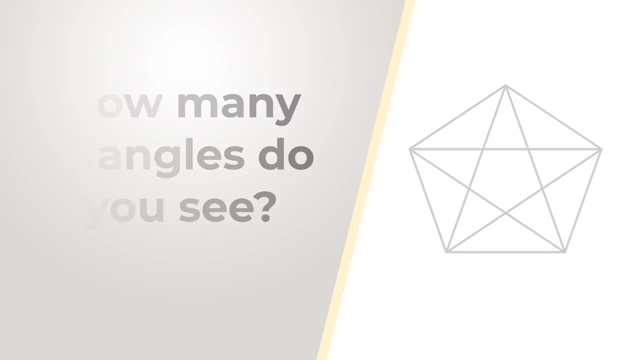 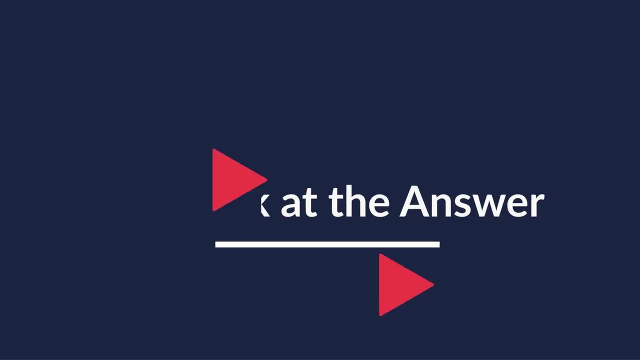 to consider the possibility of one shape being inside the other. Now let's continue to see if we can solve this challenge and get to the correct solution together. It is mind-boggling, but there are 35 triangles here. Can you believe? it Certainly was a huge surprise to me, as I was. 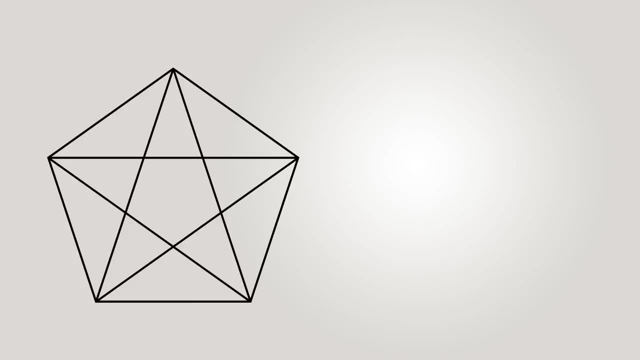 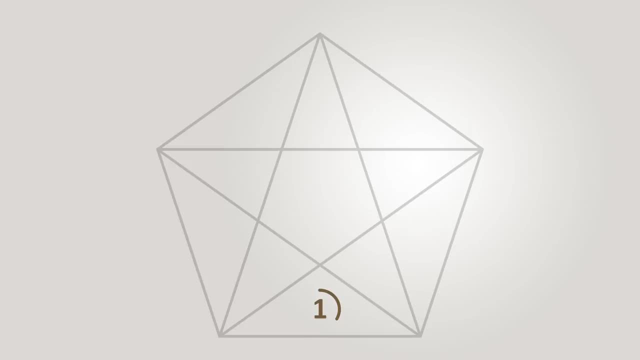 discovering them. Let me draw all of them for you. I will start by drawing small border triangles. There are 10 of them. Please count with me: 1,, 2,, 3,, 4,, 5,, 6,, 7,, 8,, 9, and 10.. Now let's. 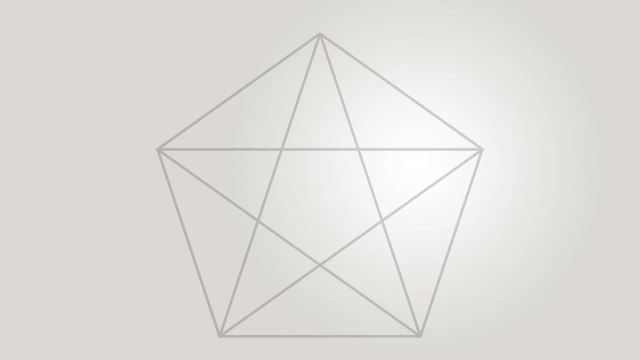 do next 10 triangles: 11,, 12,, 13,, 14,, 15,, 16,, 17,, 18,, 19,, 20,, 21,, 22,, 23,, 24,, 25,, 26,, 27,, 28,, 29,, 30,. 30,, 31,, 32,, 34,, 35,, 36,, 39,, 40,, 41,, 42,, 35,, 41,, 42,, 43,, 44,, 45,, 46,, 47,, 48,, 49,, 50,, 51,, 18,, 19,, 20.. 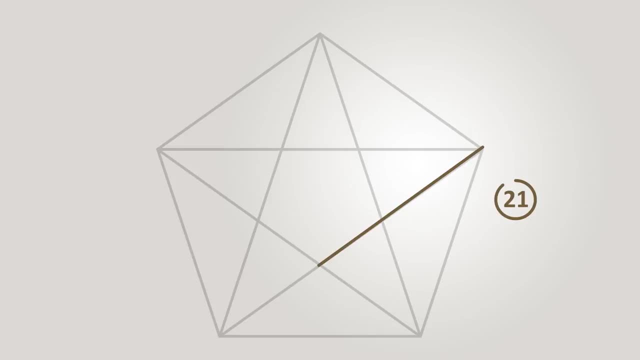 And now let's do next 5.. 20. 2, 2, 2, 3, 3.. Then let me count to see if anybody came up with a good one Under 1,, 2, 3, 3.. Let's do next 5 with the entered numbers. 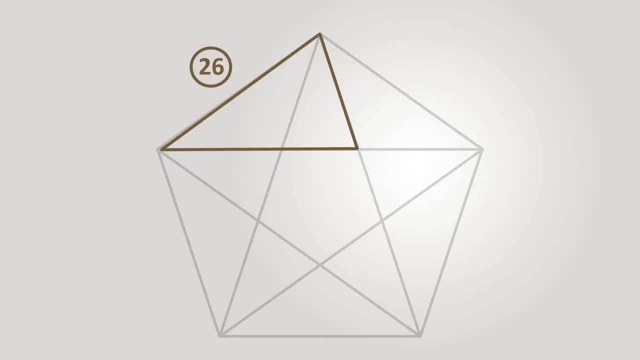 the top 5 and then the top 1 expect 2, 3,, 2, picture near basic 5eren 25.. Let me add all the numbers. Let's do. an asked Jacqueline b��us 15 migration train and 32,, 33,, 34, and the last one is 35. 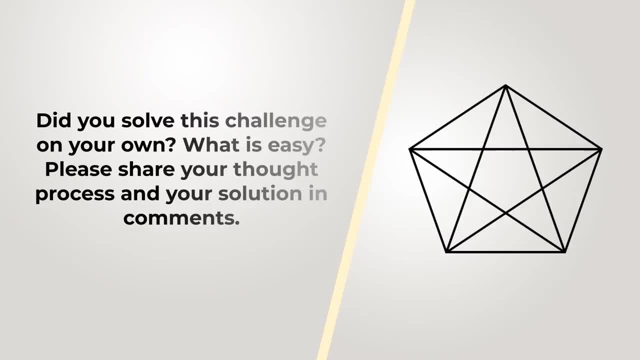 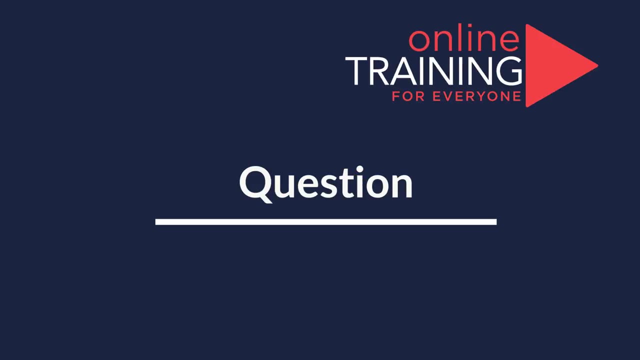 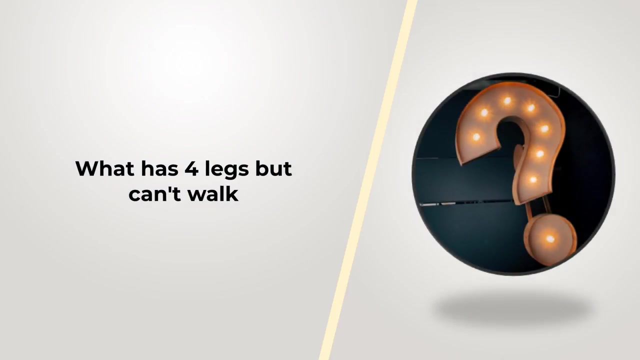 Do you think we missed any? Please make sure to leave your comment and let us know if there is even more. Hopefully you nailed this question and now learned how to answer similar questions on the test. Here is the question which tests your understanding of English language- your vocabulary as well. 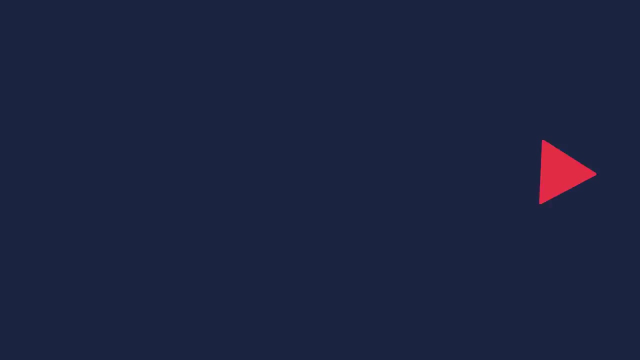 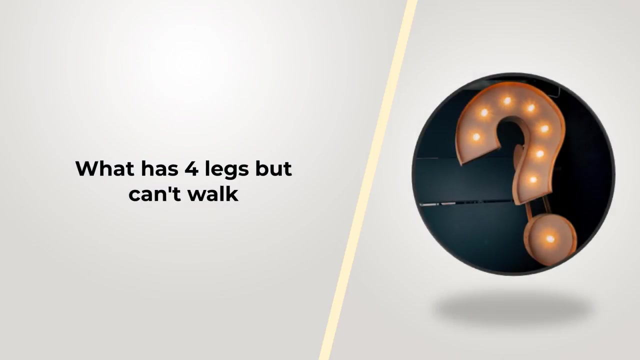 here is the question which tests your understanding of english language, your vocabulary as well as your ability in logical reasoning: what has four legs but can't walk? do you think you know the answer? now might be a good time to pause this video to see if you can. 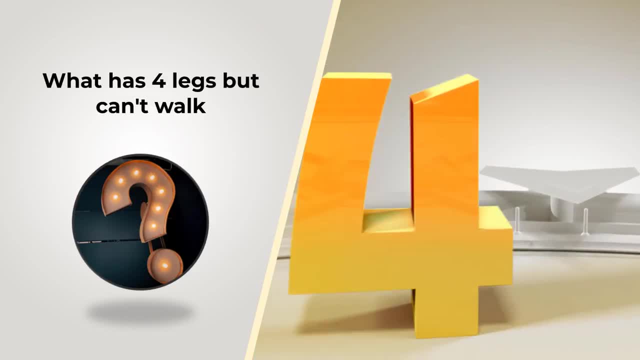 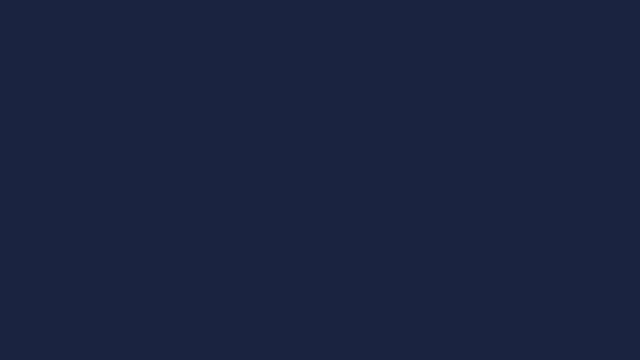 come up with the answer. do you think you found the answer? let me give you a quick hint: think out of the box and let's get started and think of not necessarily something that walks. did you figure it out? let's continue to see how we can solve this challenge and get to the correct solution together, as you might have figured it. 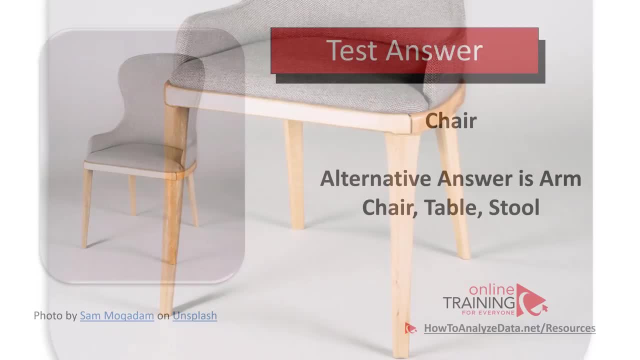 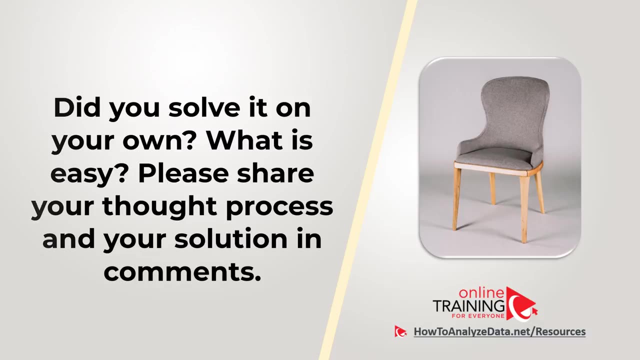 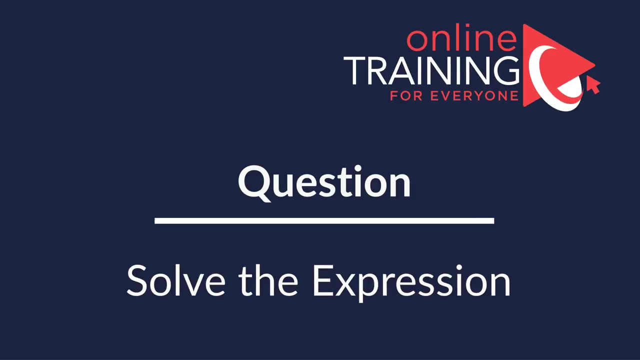 the answer is chair and the alternative answer could be armchair, table or stool. hopefully you figured it out on your own and now know how to answer similar problems on the test. here's the interesting question, which is easy to to understand but at the same time, you will have a lot of fun solving it. you need to calculate the 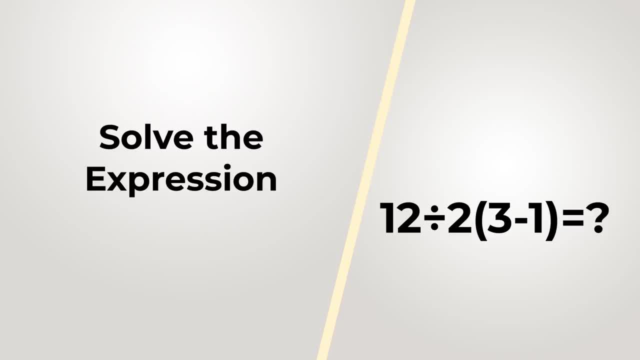 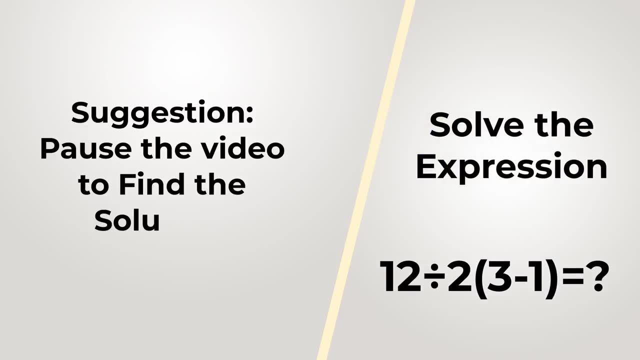 simple expression: 12 divided by 2 and then multiplied on the value in parentheses, which is 3 minus 1.. take a look closely and see if you can come up with the answer. there are three operations here: division, multiplication and subtraction. all you need to determine is which one to do first. 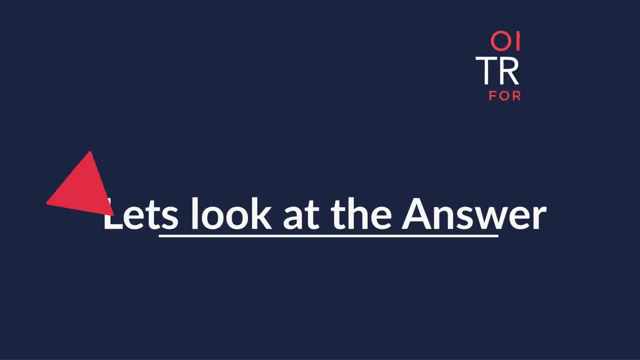 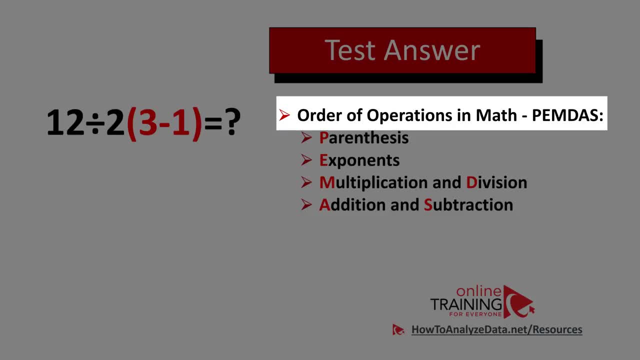 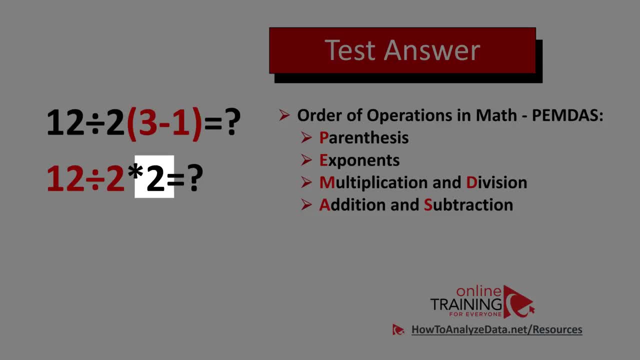 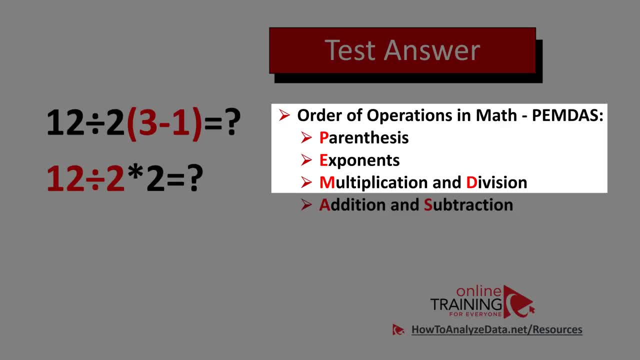 tells us that we need to do multiplication and division. but what order doesn't mention is that we need to do it from left to right. and, what's interesting, the acronym itself is a little bit confusing, because it shows multiplication first and then division, but in our case we need to do division. 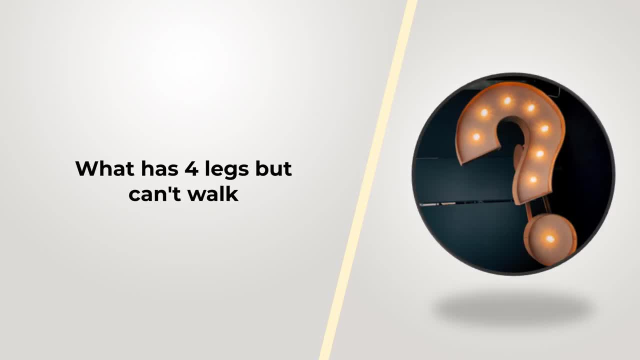 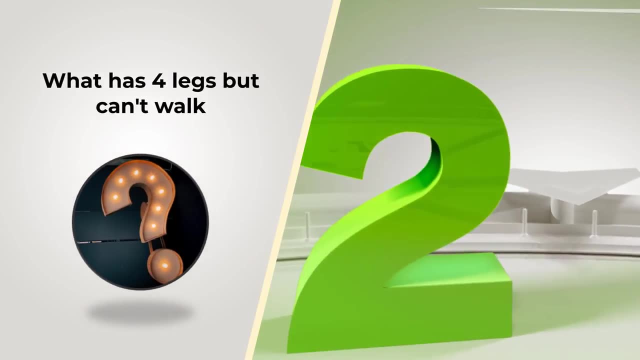 as your ability in logical reasoning. What has four legs but can't walk? Do you think you know the answer? Now might be a good time to pause this video to see if you can come up with the answer. Do you think you found the answer? 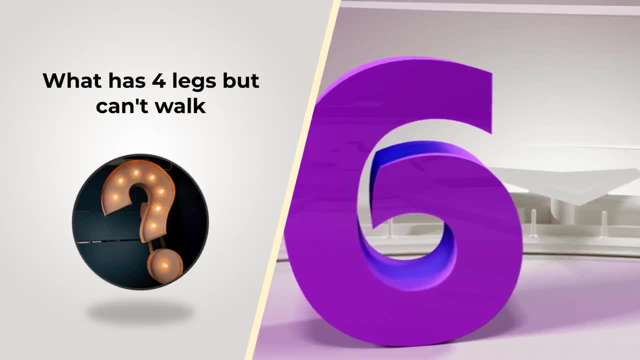 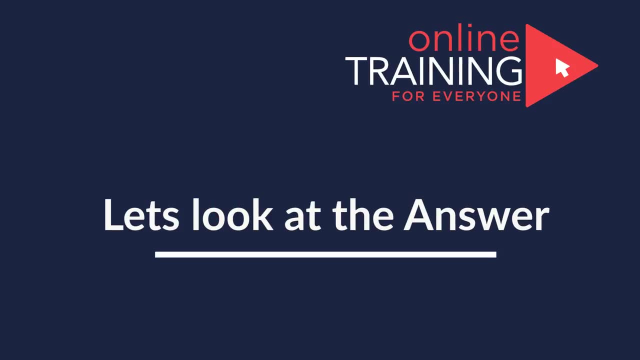 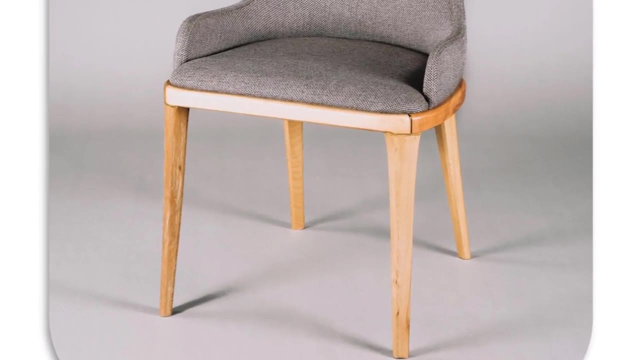 Let me give you a quick hint. Think out of the box and think of not necessarily something that walks. Did you figure it out? Let's continue to see how we can solve this challenge. As you might have figured it, the answer is chair and the alternative answer could. 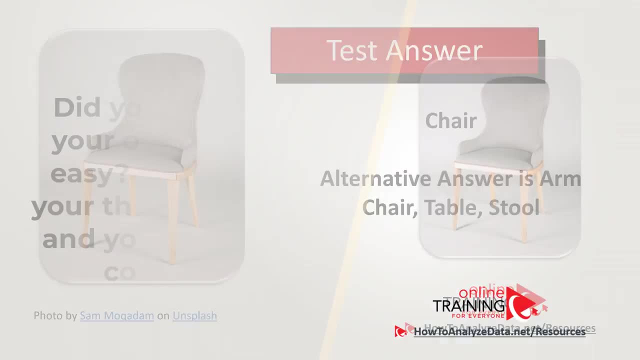 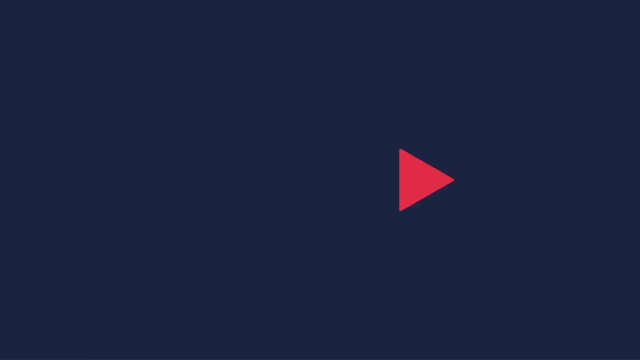 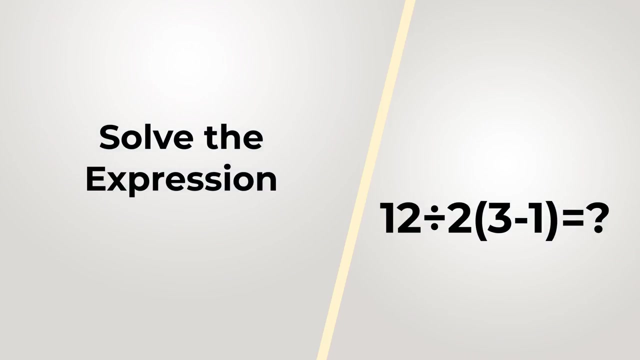 be armchair, table or stool. Hopefully you figured it out on your own and now know how to answer similar problems on the test. Here is the interesting question, which is easy to understand but at the same time, you will have a lot of fun solving it. 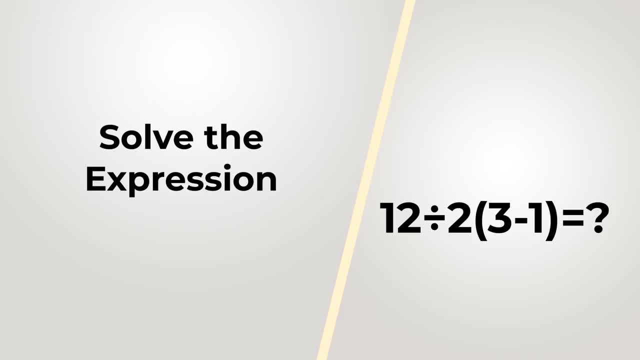 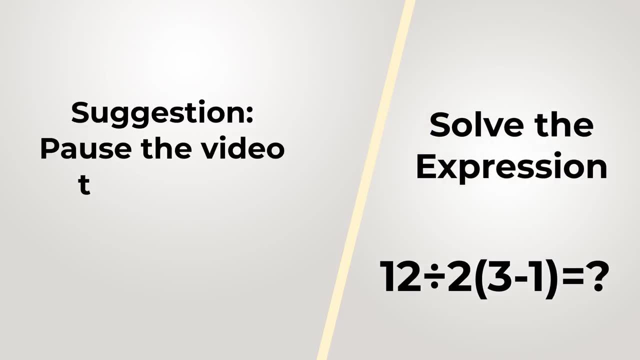 You need to calculate this simple expression: 12 divided by 3.. Divided by 2 and then multiplied on the value in parentheses, which is 3 minus 1.. Take a look closely and see if you can come up with the answer. 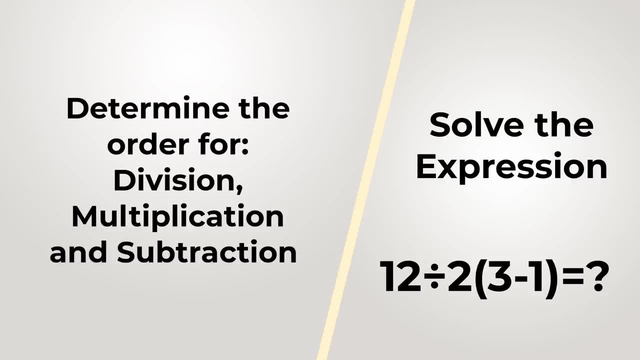 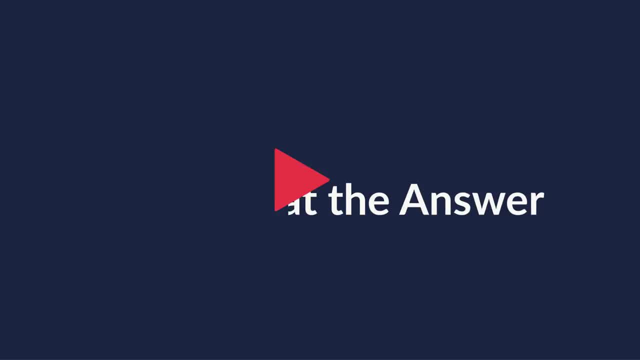 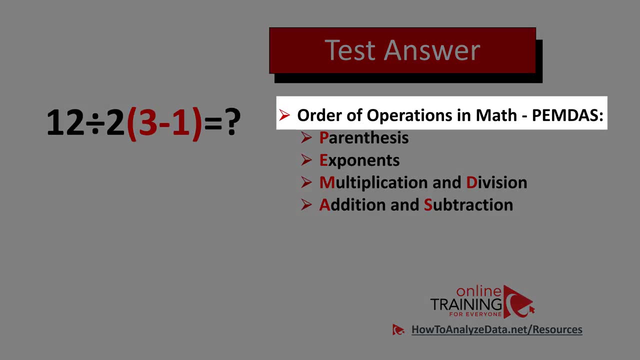 There are three operations here: division, multiplication and subtraction. All you need to determine is which one to do: first, second and third. Do you think you know the answer? Let's continue and get it solved together. The order of operations in math tells us that the first and the second are the same. 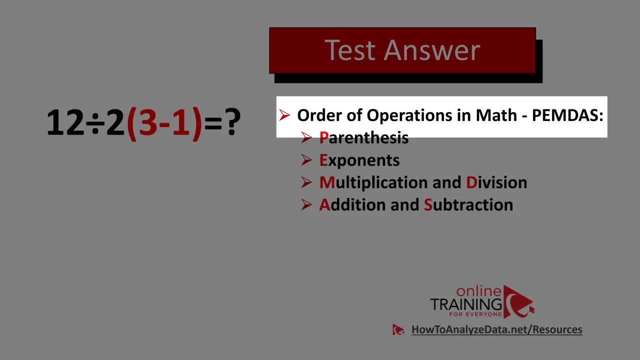 The order of operations in math tells us that the first and the second are the same. The order of operations in math tells us that the first and the second are the same. The first expression we need to solve is in parentheses. We first need to calculate 3 minus 1.. 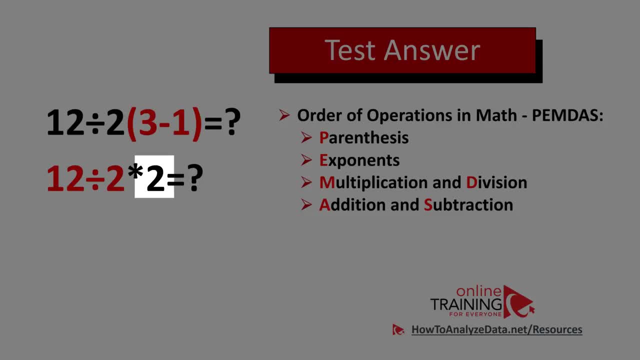 And obviously the answer is 2.. The big question is: what do we do next? The order PEMDAS tells us that we need to do multiplication and division, But what order doesn't mention is that we need to do it from left to right? 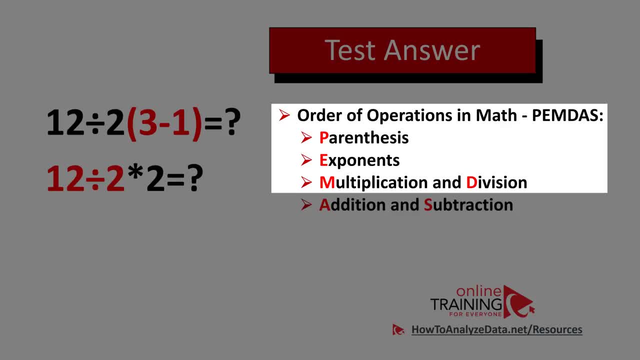 And what's interesting, the acronym itself is a little bit confusing because it shows multiplication first and then division. But what's interesting is that the acronym itself is a little bit confusing because it shows multiplication first and then division. But what's interesting is that the acronym itself is a little bit confusing, because it shows multiplication first and then division. 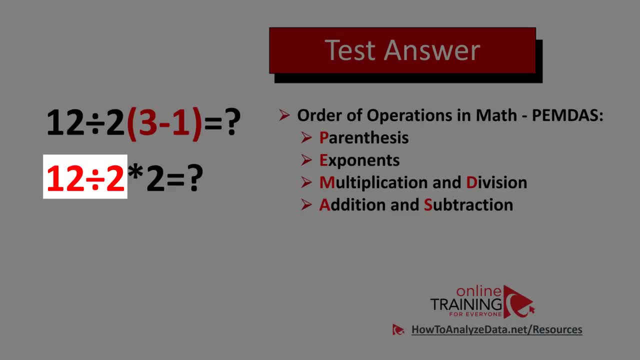 But in our case we need to do division first, and divide 12 by 2, and then do multiplication. Once we divide 12 by 2, we get to 6, and the final expression we need to solve would be 6 multiplied by 2.. 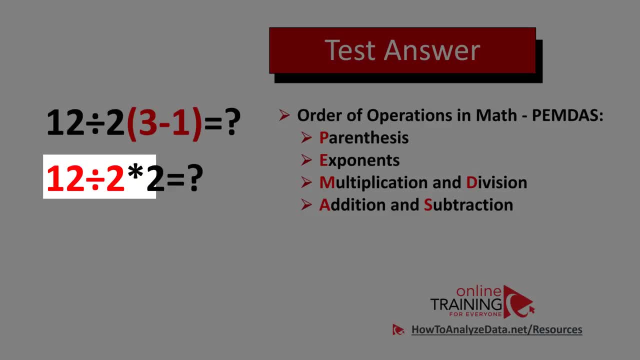 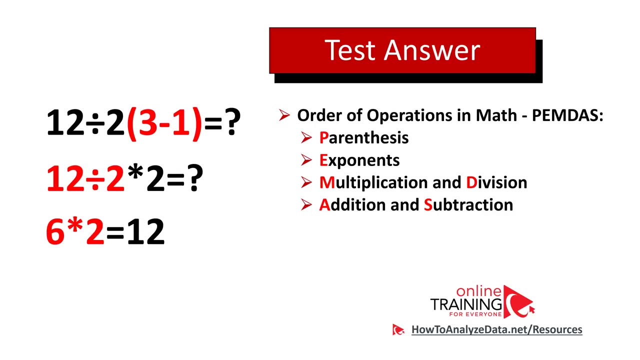 first and divide 12 by 2 and then do multiplication. once we divide 12 by 2, we get to 6, and the final expression we need to solve would be 6 multiplied by 2. so the correct answer here is 12. let me give you a quick hint, even if you don't. 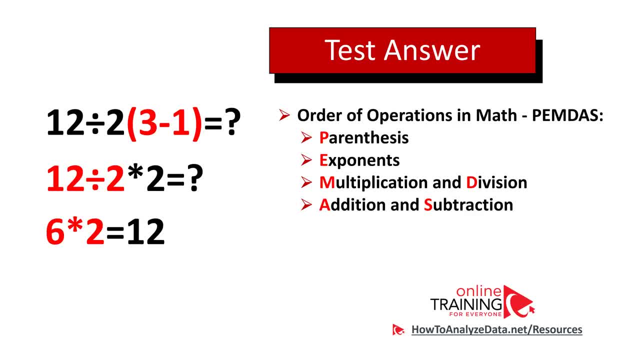 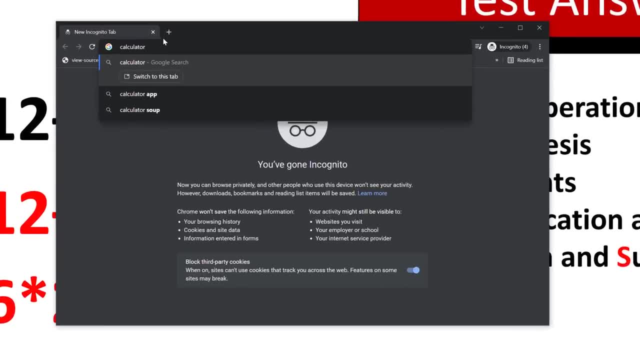 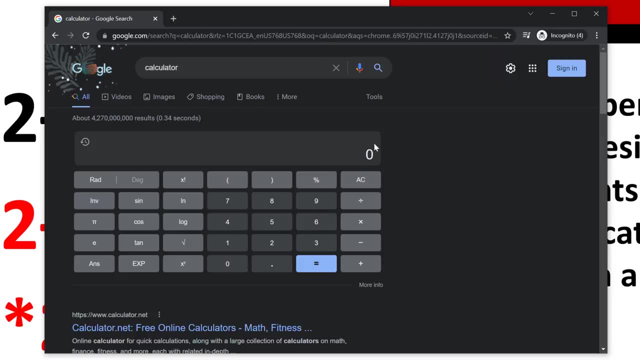 know the answer. you can always use a calculator. most modern calculators do support expressions. let me demonstrate for example. if you type calculator in Google, it shows the calculator which you can use to solve the expressions. you can preview expression and once you keep the equal sign, it calculates it for. 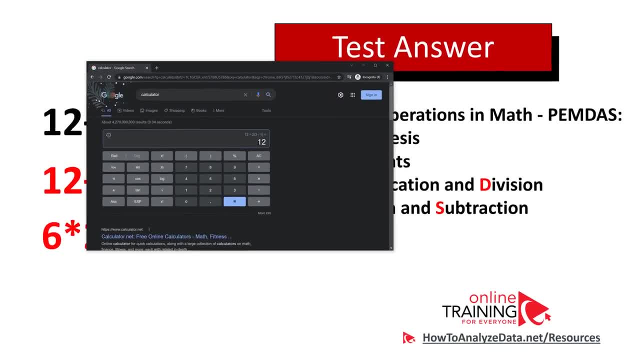 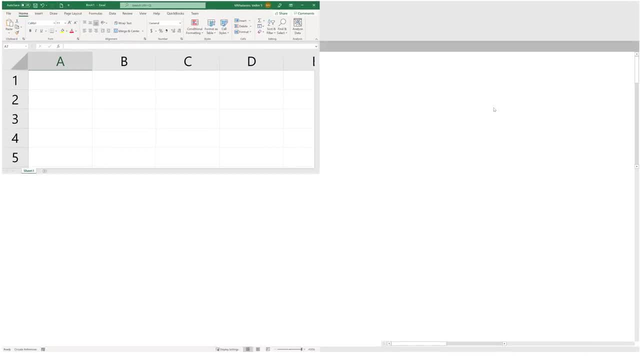 you and you can use it to solve the expressions. you can preview expression and once you hit the equal sign, it calculates it for you and you can see that the correct answer here is 12. another alternative is to use Microsoft Excel, which is available on almost any Windows machine. here you can. 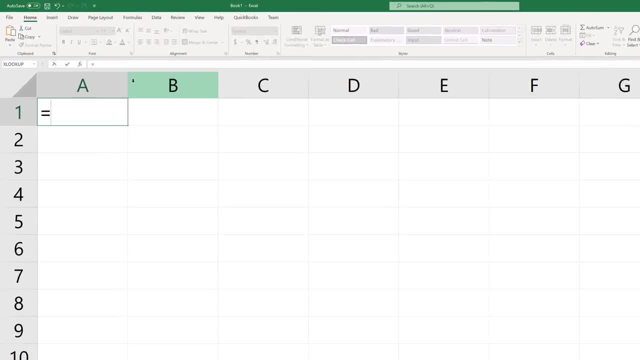 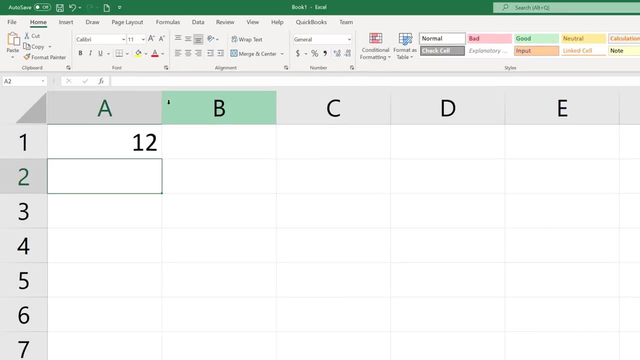 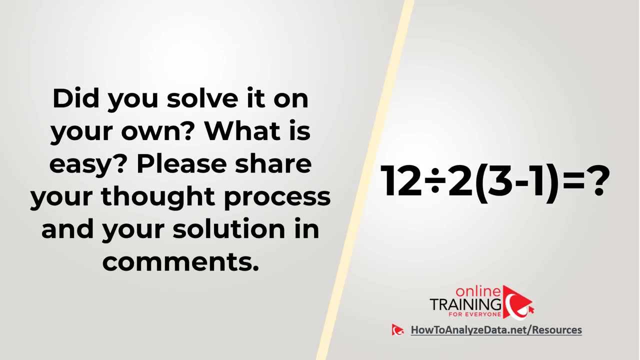 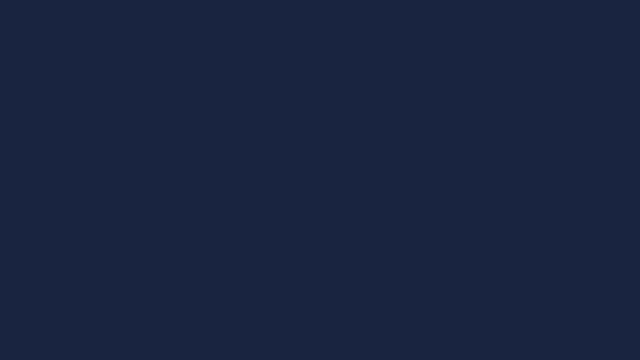 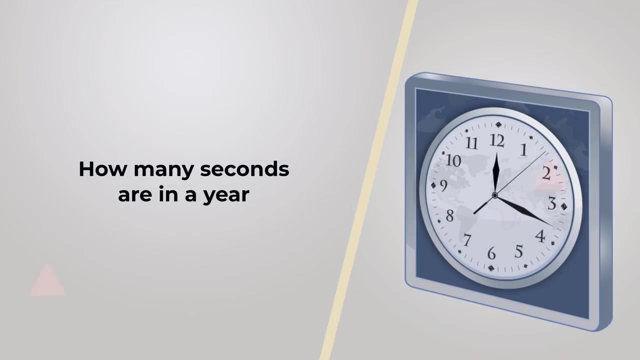 enter the expression right inside any cell in Microsoft Excel will perform the calculations. so did you solve this challenge on your own? was it easy for you? please share your thought process and your solution in the comment section of this video. I had this question being asked as part of consulting job. 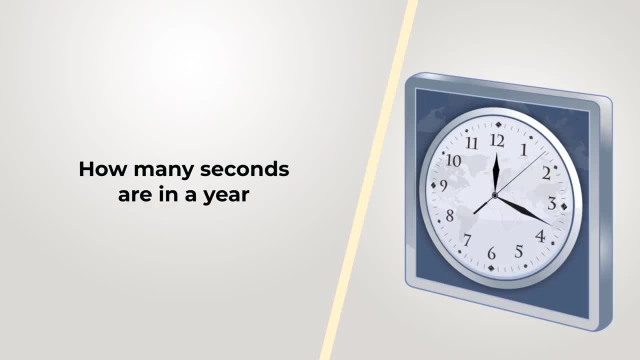 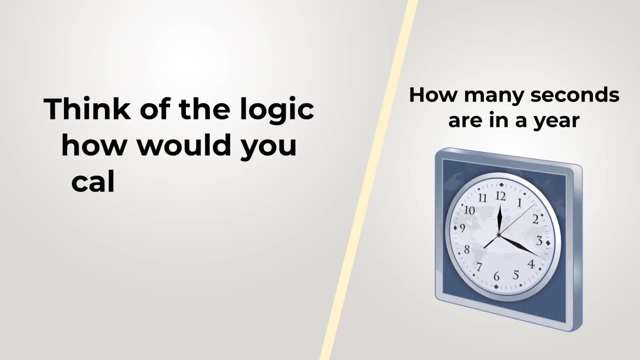 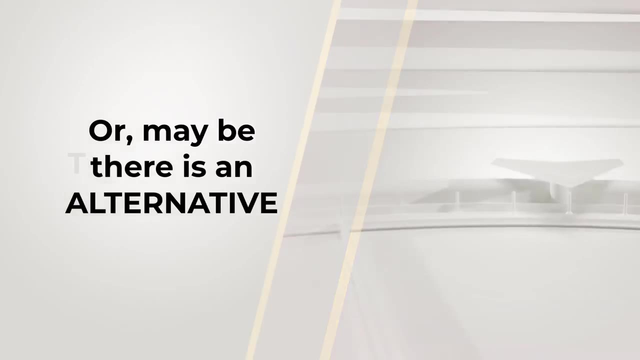 interview. how many seconds are there in the year? take a look at the picture. it might give you a hint. do you think you know the answer? think of the logic. how would you calculate how many seconds are there in the year? or maybe the? there is an alternative. always try to think out of the box. this would be my. 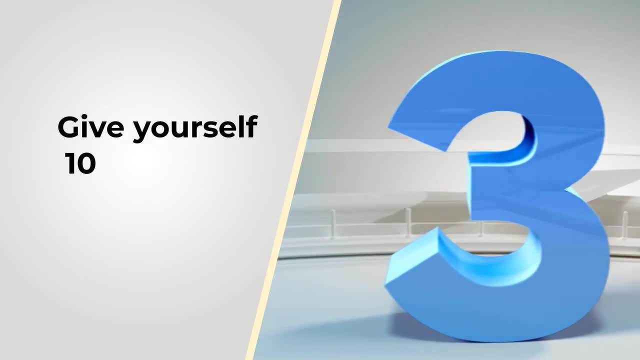 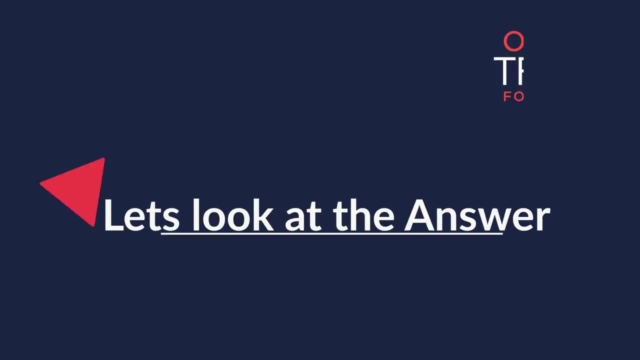 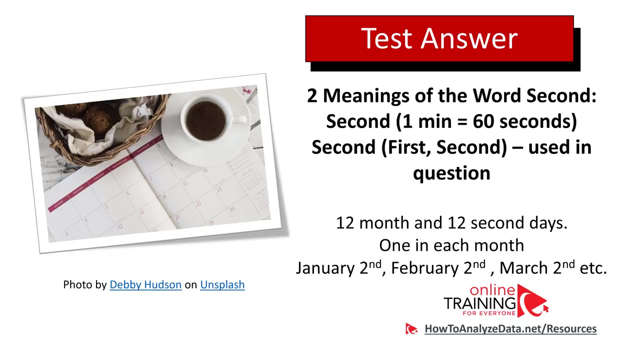 hint to you and give yourself 10 to 15 seconds. this is as much time as you might get answering these types of questions in the test. now let's continue and get to the correct solution together. obviously, this is a tricky question and it challenges you in understanding of the word. second, there are two meanings. 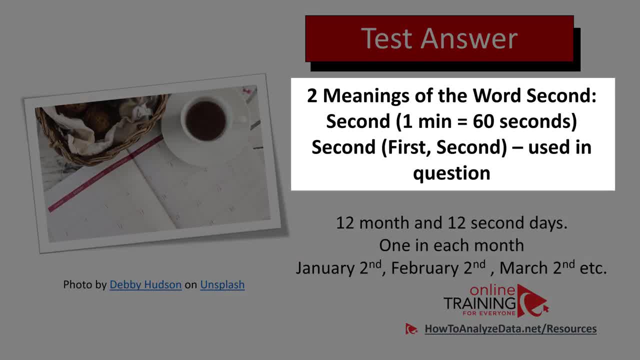 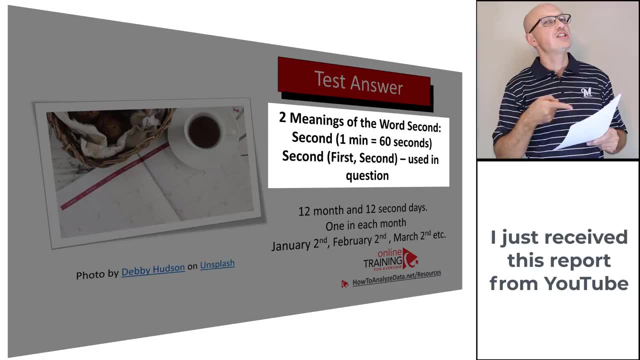 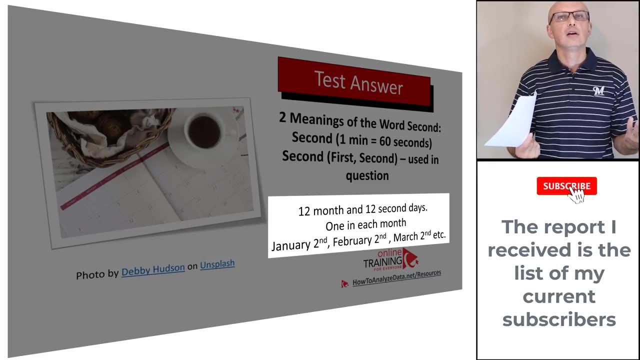 in the word second one is second. for example, one minute has 60 seconds, but second one is second, where you have sequence of first and second and the second meaning of the second is used in this particular question. so if we go back to the question, in the year there are 12 months. 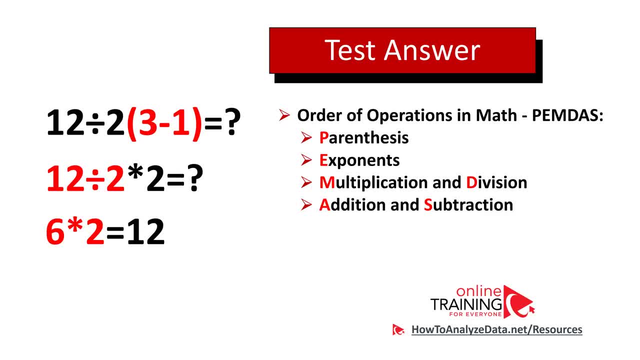 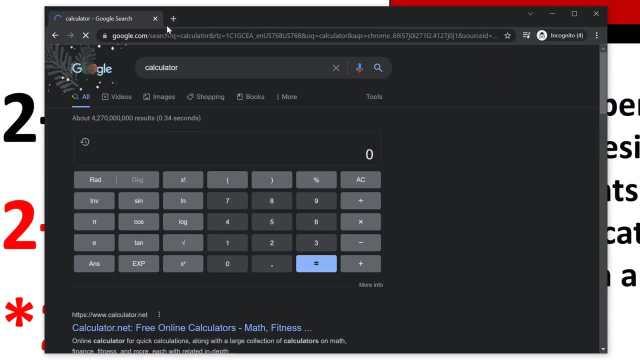 So the correct answer here is 12.. Let me give you a quick hint, Even if you don't know the answer. you can always use a calculator. Most modern calculators do support expressions. Let me demonstrate, For example. if you type calculator in Google, it shows the calculator which you can use to solve the expressions. 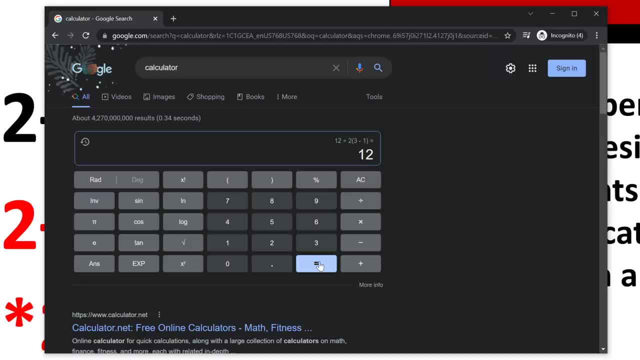 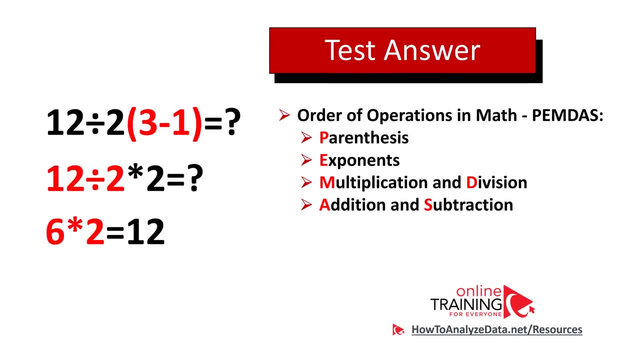 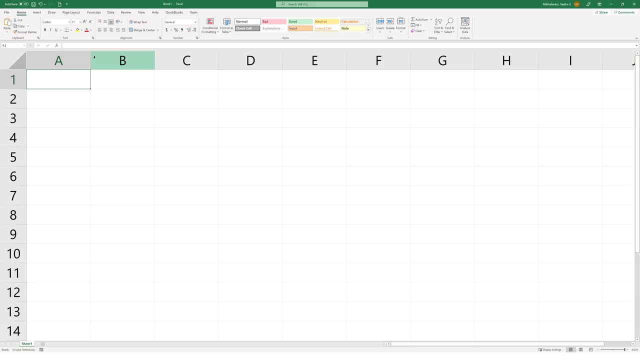 You can preview expression and once you hit the equal sign, it calculates it for you And you can see that the correct answer here is 12.. Another alternative is to use Microsoft Excel, which is available on almost any Windows machine. Here you can enter the expression right inside any cell. 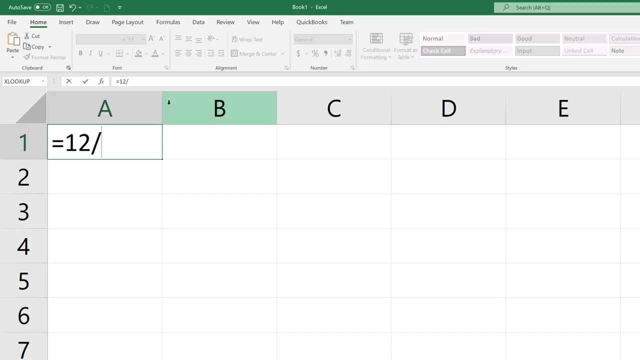 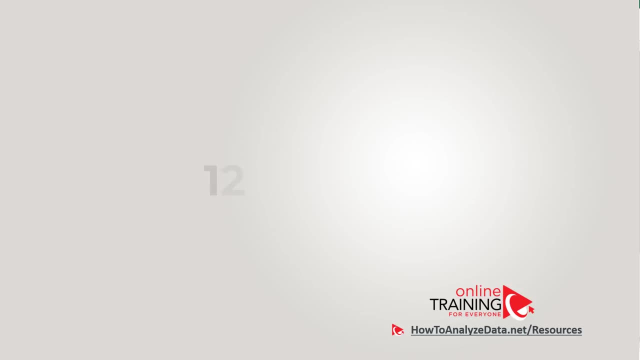 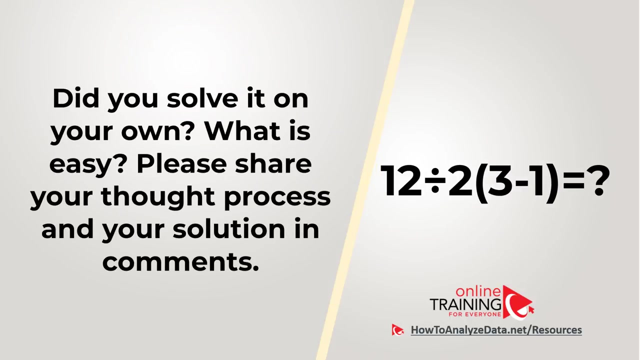 And Microsoft Excel will perform the calculations. So did you solve this challenge on your own? Was it easy for you? Please share your thought process and your solution in the comments section of this video. I had this question being asked as part of a question. 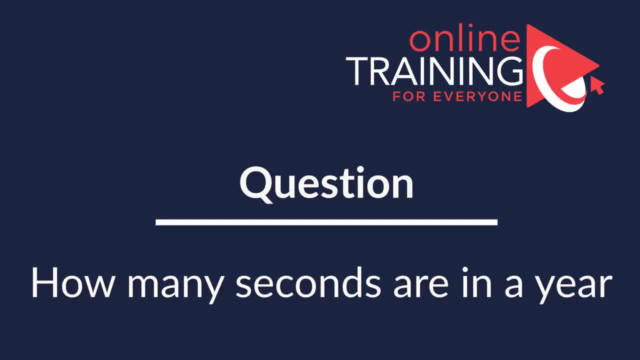 I'm not sure if this is the right way to do it, but I think it's a good way to do it. If you have any questions, please feel free to ask them in the comments section of this video. If you have any questions, please feel free to ask them in the comments section of this video. 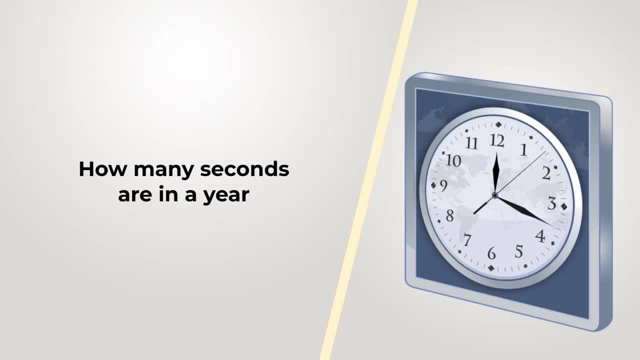 But let's start with the domiciled version. Here you will find the result of your test. I named the test as part of a consulting job interview. How many seconds are there in the year Xi k hay, Day two. Good, Take a look at the picture. 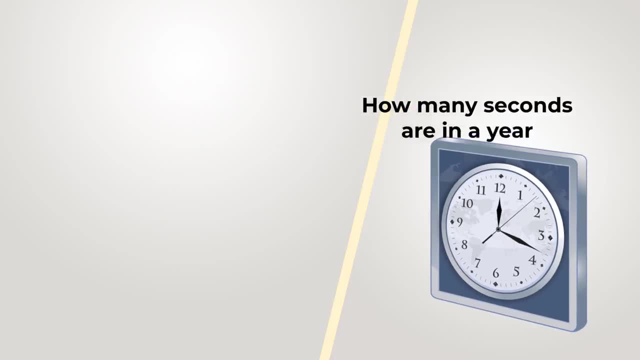 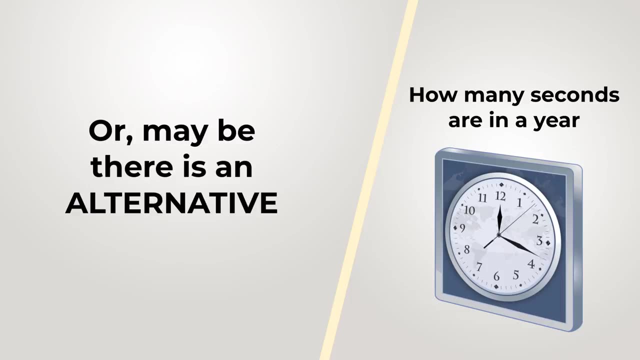 It might give you a hint. Do you think you know the answer? Think of the logic. how would you calculate how many seconds are there in the year? Or maybe there is an alternative. Always try to think out of the box. This would be my hint to you. 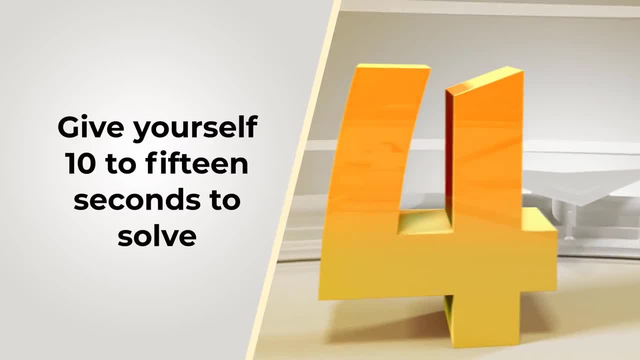 And give yourself 10-15 seconds. This is as much time as you might get answering these types of questions in a test. So if you have any questions about electronic tools, dont hesitate to write to us via the chat below, so that we can hear you next time on Wayne Tech Content. 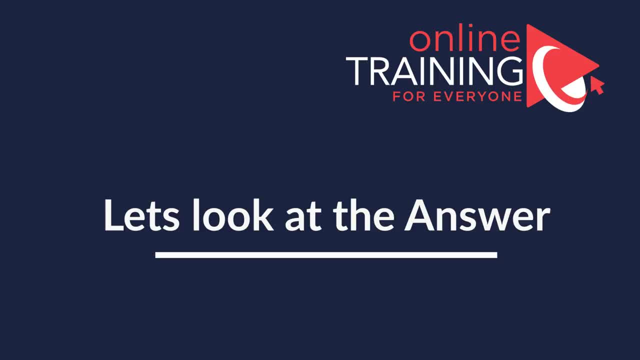 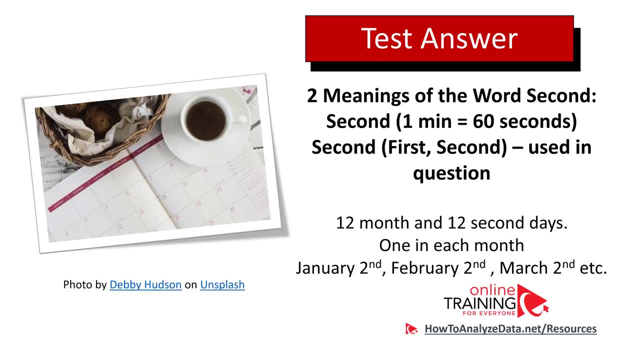 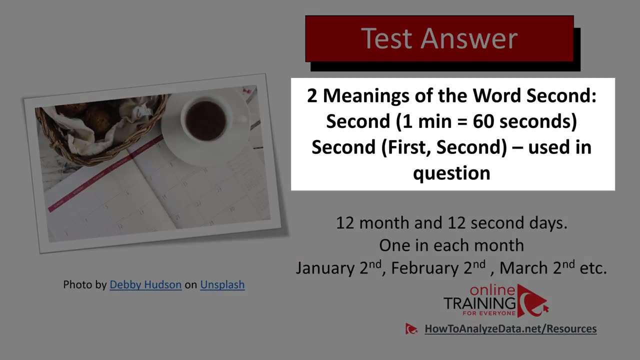 now let's continue and get to the correct solution together. obviously this is a tricky question and it challenges you in understanding of the word second. there are two meanings in the word second. one is second. for example, one minute has 60 seconds, but second. one is second, where you have sequence of first.